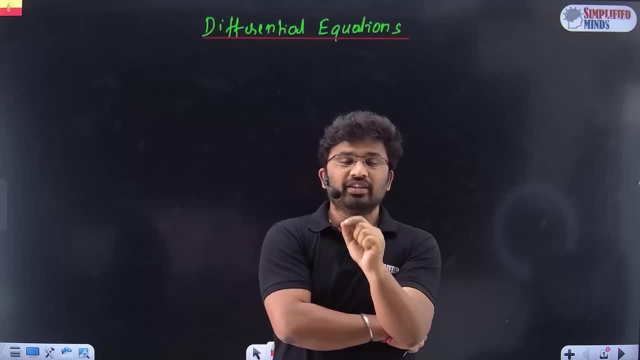 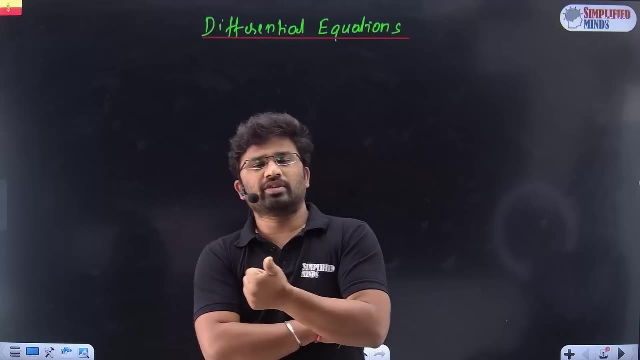 I want you to score full, out of full in the Calculus. So now in the last chapter of Calculus, Differential Equations. In this lecture we will discuss about Basics. What is Differential Equations? basically, What is the general solution? 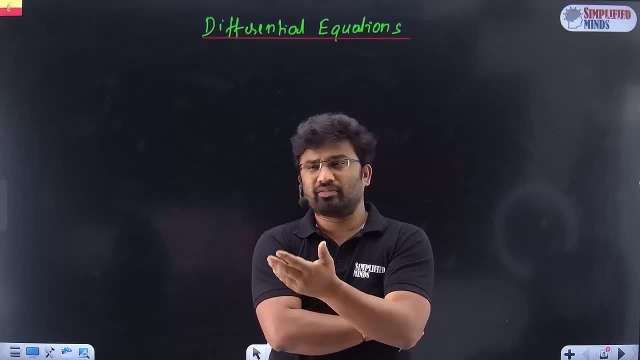 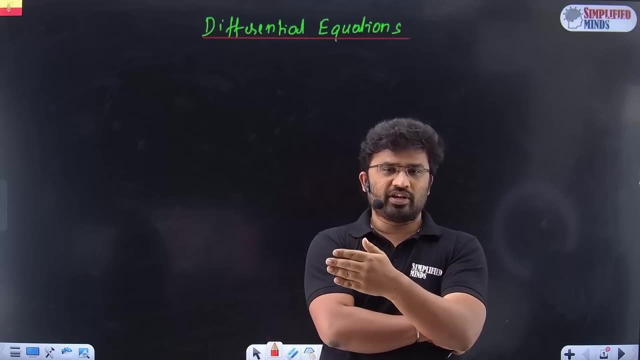 What is the particular solution? What is the general solution? What is the order degree? We will discuss the basics of Differential Equations. In the Admin you have something called as Forming Differential Equations, But as per the new rules, NCRD syllabus has deleted the Forming Differential Equations. 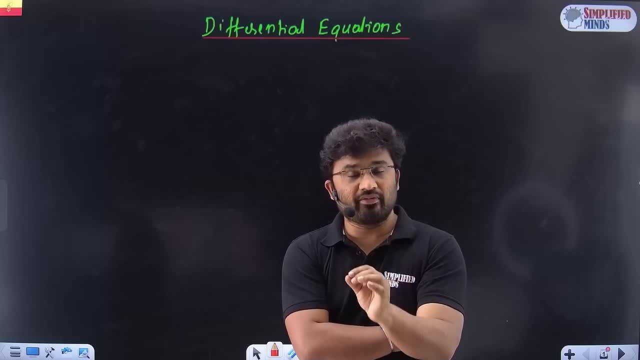 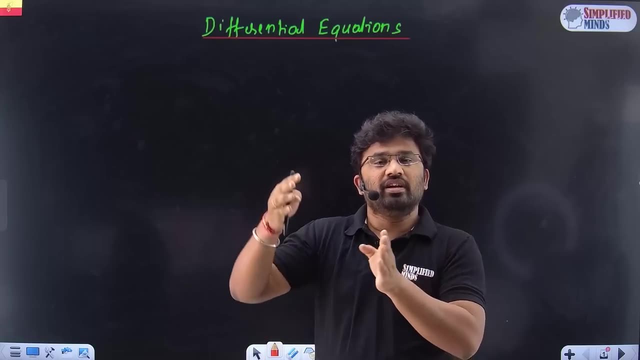 In the Admin we have Solving Differential Equations, Which is very, very important for you In the Board Exams. you will hear about it And Differential Equations is the main, major heart of Differential Equations. Solving Differential Equations. 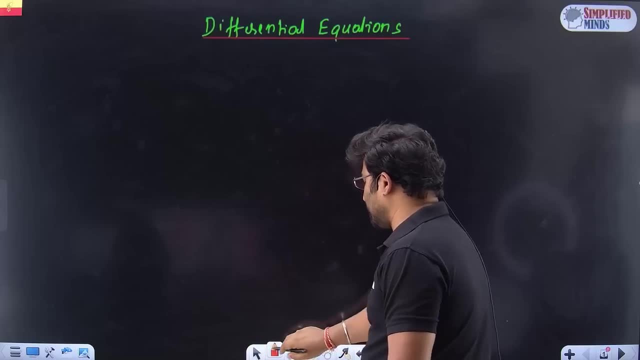 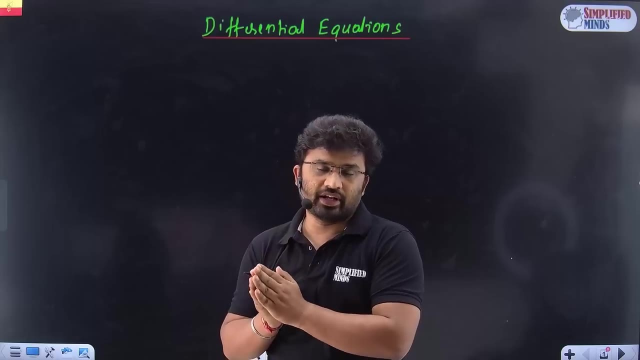 We have different methods: Linear Method, Homogeneous Method. In the Admin you have Variable Supplemental Method. We will discuss that in a different lecture. First we will understand Basics. That is very, very important. Always you have to go in your order. 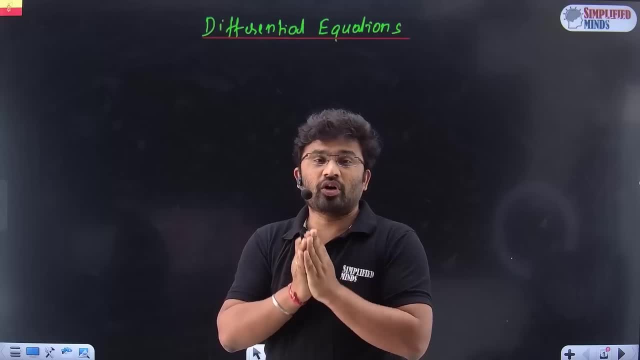 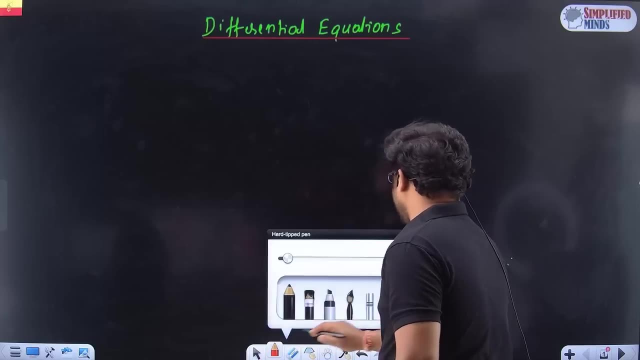 When I say Calculus, you have to understand it, You have to go in your order. I hope you are loving Calculus And don't forget to comment: Calculus is Love. Then we will go for one lecture. First, what is Differential Equation? 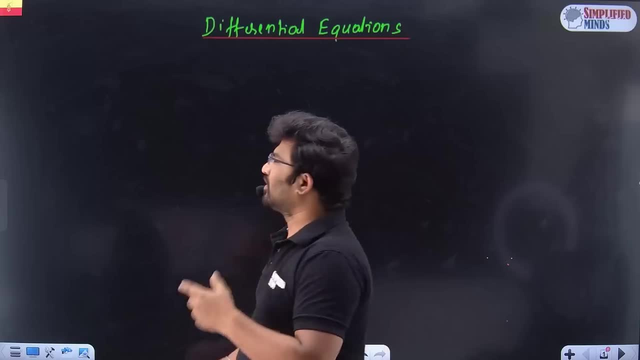 Sir, it is very simple. What is Equation In Equation? you know it is simple. For example, you have already learnt it: x square plus 10x. you know. For example, it is like this: For example, 10x plus 6 must be equal to 0.. 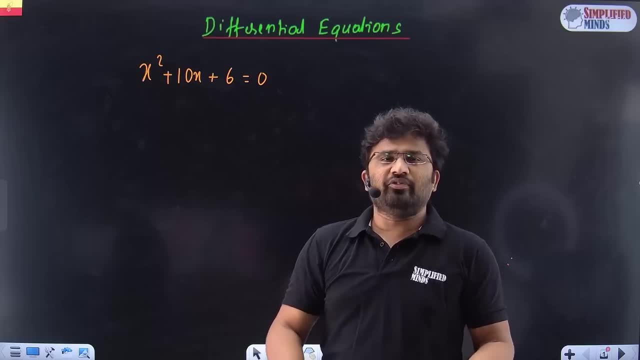 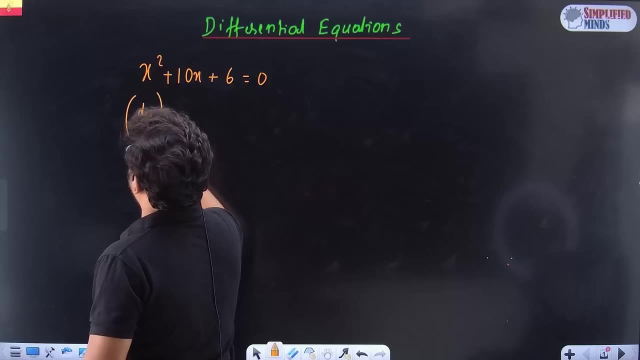 So this is an Equation That is a Differential Equation. In Differential Equation, you know, In terms of differentiation, there is dy by dx. So dy by dx is like this: Something square In that, something like maybe 10 into dy by dx. 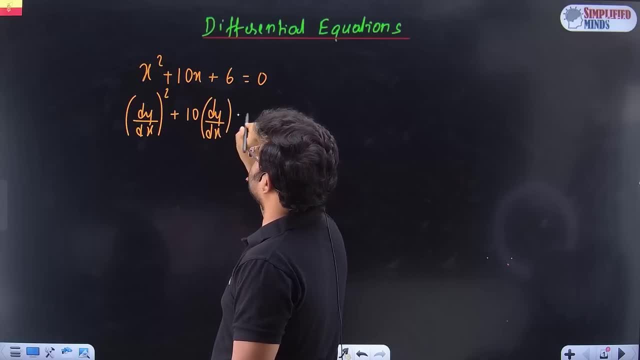 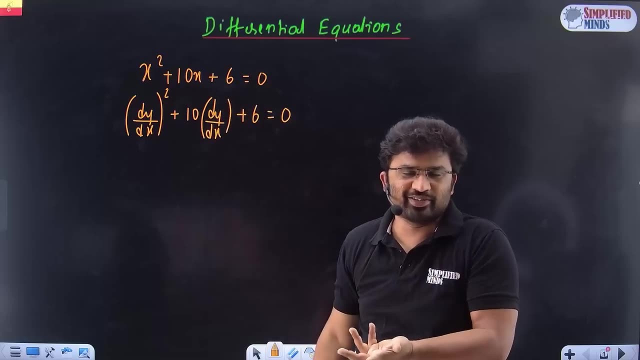 10 into dy by dx. This is a Differential Equation. 10 into dy by dx, plus 6 must be equal to 0. This is a Differential Equation. So this is a Normal Equation. Here it is a Differential Equation. 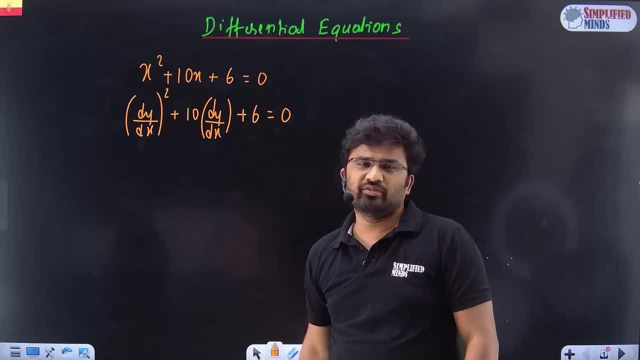 So this is a Differential Equation As of now, one day. variable differentiation you always do only with respect to dx, But when higher classes are going on, you will do with respect to dx. dy, You will do with respect to two more variables. 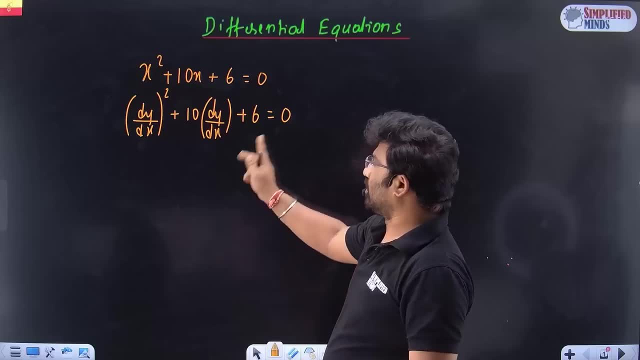 We have something called Partial Derivatives. So first you have to understand this, First this is only one thing. So if you find a solution for this, if you find a solution for this, you will get some x is equal to some constants, right? 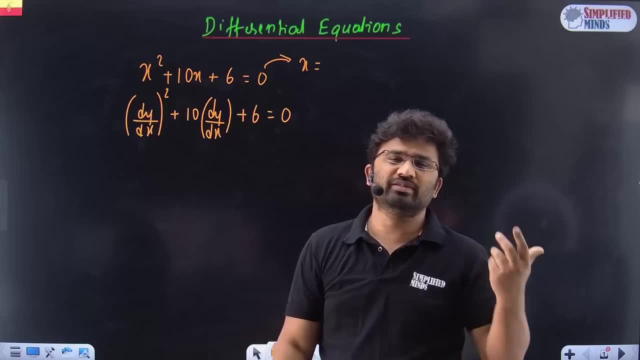 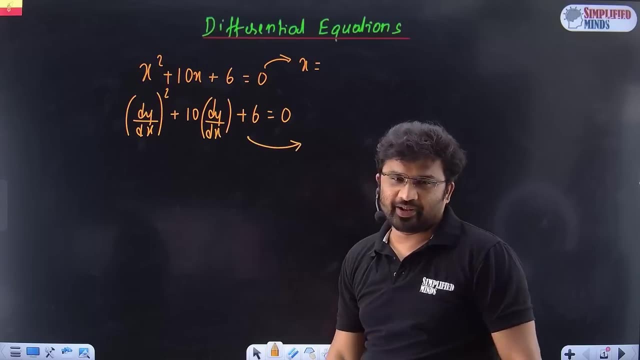 If x is equal to 5,, 6,, any real numbers will come. You are already learning in lower classes. Now, similarly, if I find a solution for this, the solution of a Differential Equation, if you find a solution for a Differential Equation, 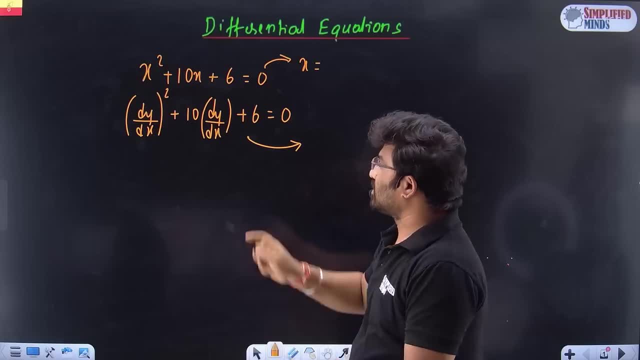 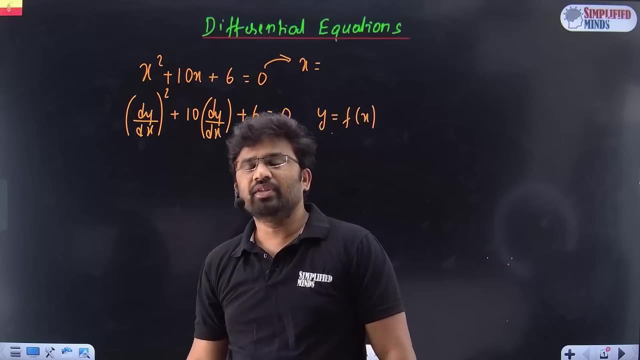 that too will become a function. So, if you find a solution for this, you will get something like y is equal to something, f of x Or some constant. you will have some arbitrary constants. So y is equal to f of x. 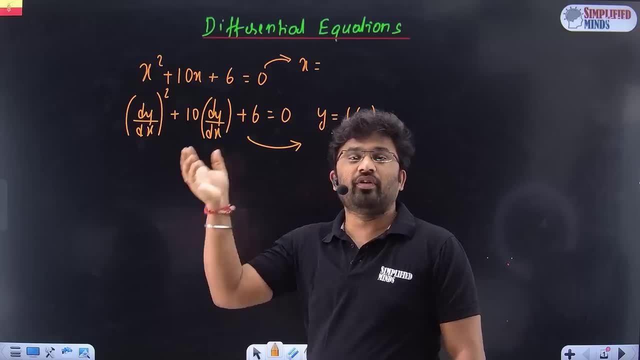 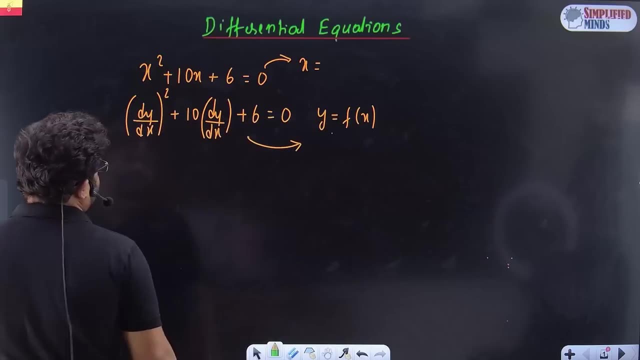 So solution of a Differential Equation is also a function. It is a function. I will give you a simple example. Just understand it. See, very, very simple. For example, if I take- let us take a simple example- y is equal to: 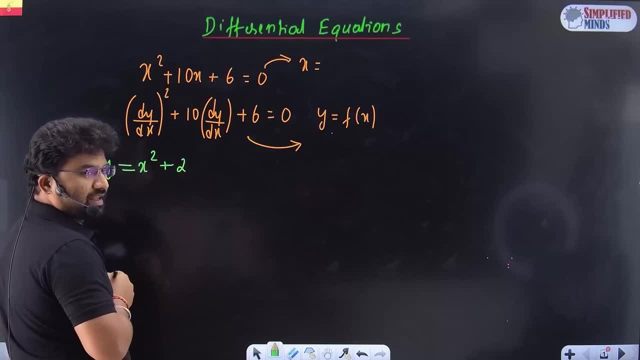 I will simply take x square plus 2.. This is an equation. Now, after differentiating this dy by dx, we will get 2x. Differentiation of 2 is 0, 2x will come. So what will I do with this? 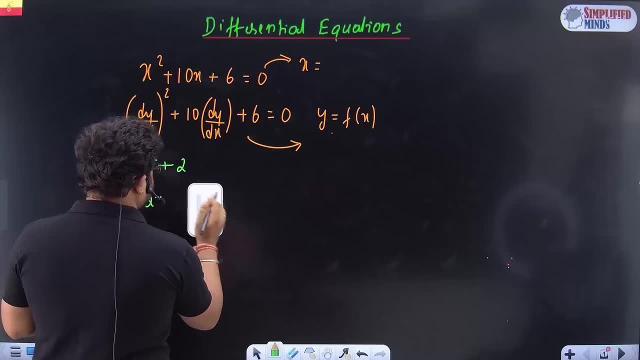 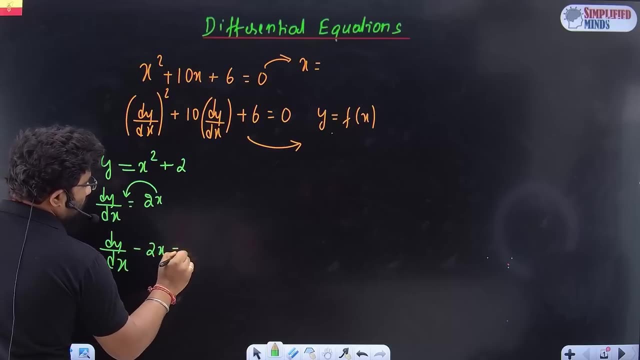 I can write this as: What will I do with this? So I will write like this: So dy by dx will come. I will shift this 2x here, Minus 2x equal to 0.. So this is a question. 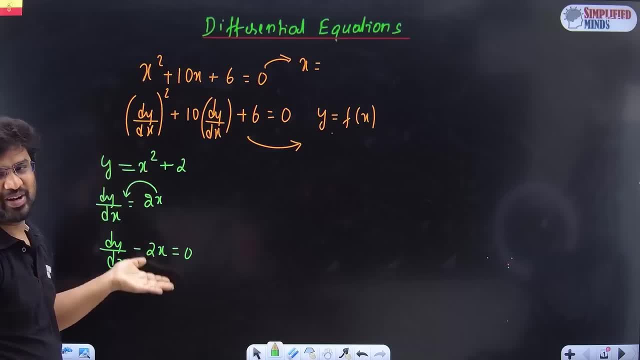 This is y is equal to x square plus 2.. We have already learned this. We have differentiated Find dy by dx. When you find dy by dx, you will get, like this, dy by dx equal to 2x. So this equation: 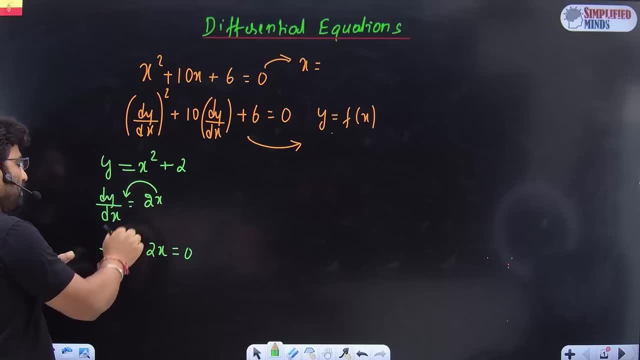 we have to equate it to something right: y equal to 0. So getting 2x this side, we got an equation. So this is the function and this was the differential equation. So what are you doing? 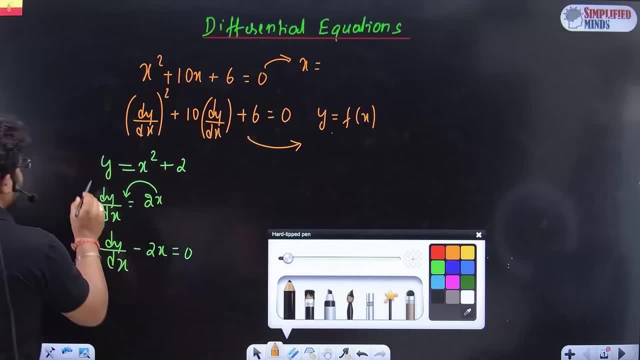 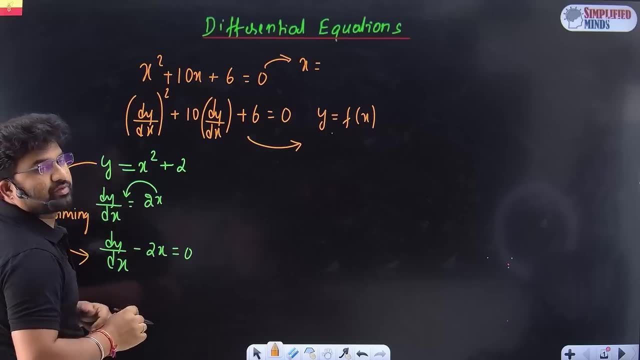 For example- from here this is only called forming differential equation- And the function given, which function is given, y is equal to x square plus 2.. For the second one, y is equal to- just you will get like something x square plus a. 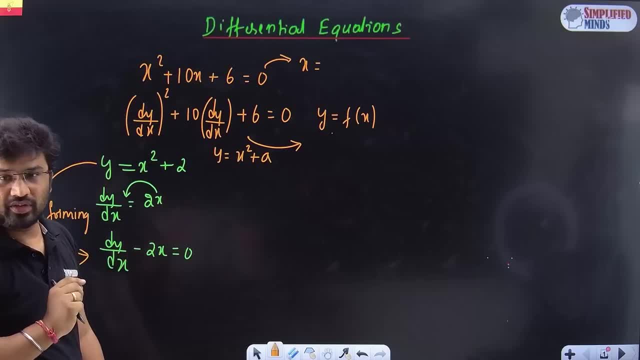 and it is given General. Or you get sin ax plus b and it is given. So some arbitrary constants are given. Why Random a, b, c, d? So if any function is given, you differentiate it right. 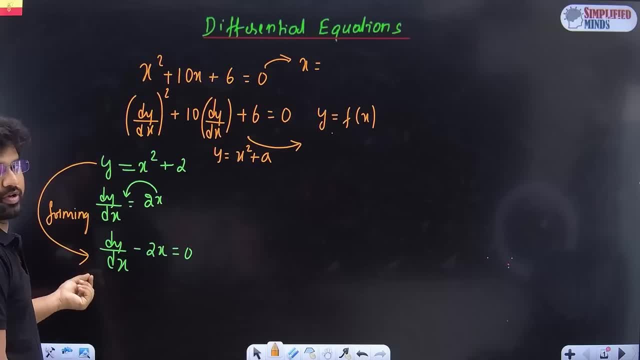 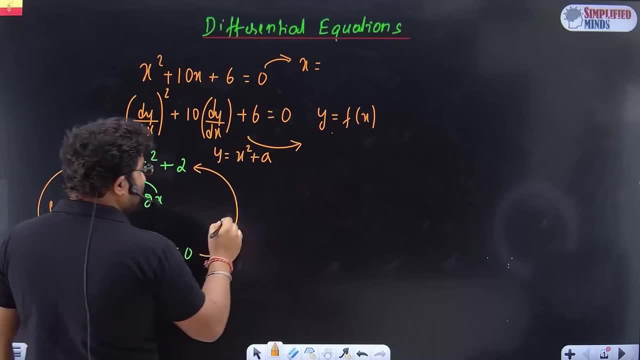 You differentiate it and eliminate that constant right That is forming differential equation. After that, you find the solution for this like this: This is the solution you find, like this. This is called a solving differential equation. Solving Solving differential equation. 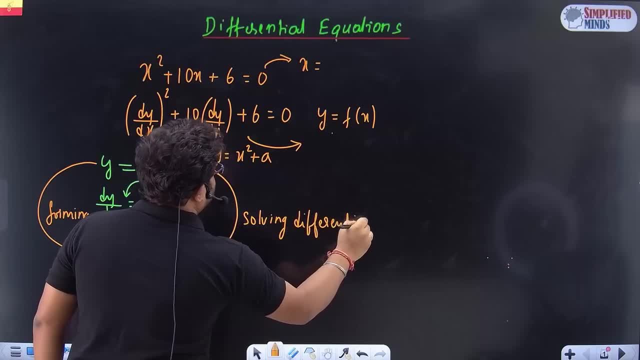 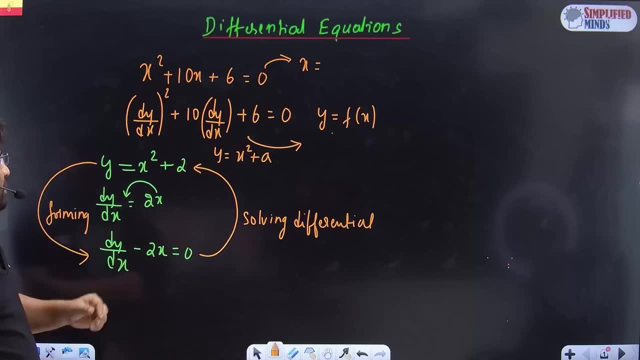 What is solving? They themselves give differential equations. They themselves give differential equations. If you solve it, ultimately you will get: y is equal to f of x. Then we have something called particular solution, general solution. I will discuss that. 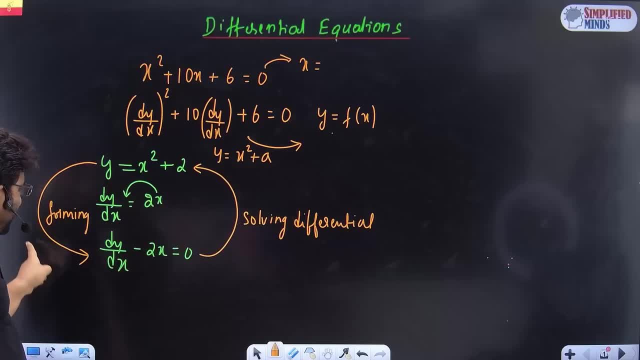 okay, Is it clear? So, forming differential equation, solving differential equation As per the new NCRT, this forming is there, But solving in this is normal guys. Is it clear? So this is called as differential equations. 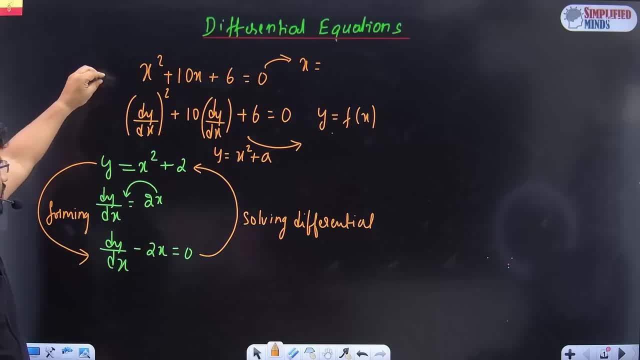 So any question given by anyone can be solved like this, And so this is a given function. One differential equation is a solution to a given function. If you find a solution to a differential equation, you will get always a. 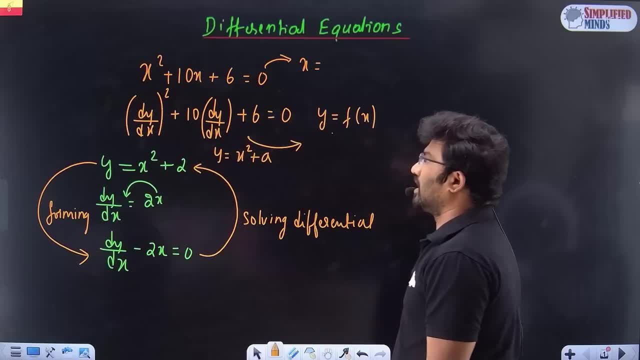 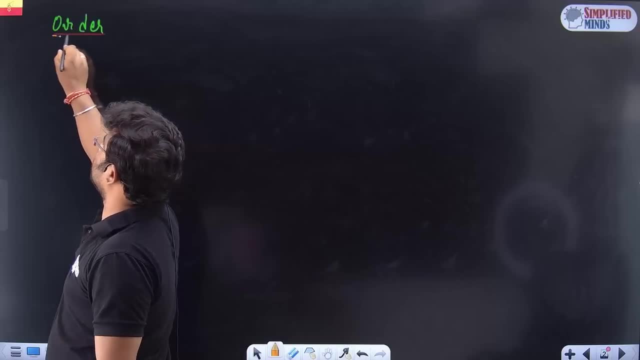 you know, y is equal to x square plus y is equal to f of x. Is it clear? This is called differential equations. I am saying it simply. Next order of a differential equation. Order is very simple. How many times did you differentiate? 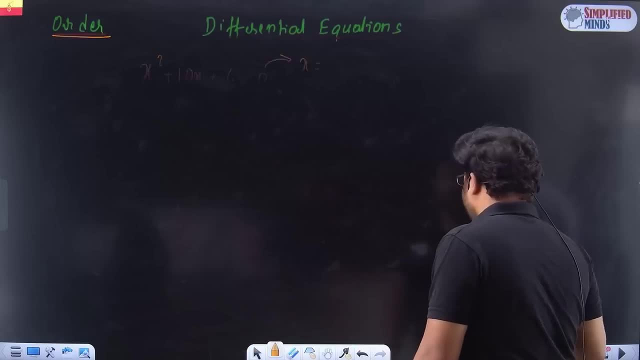 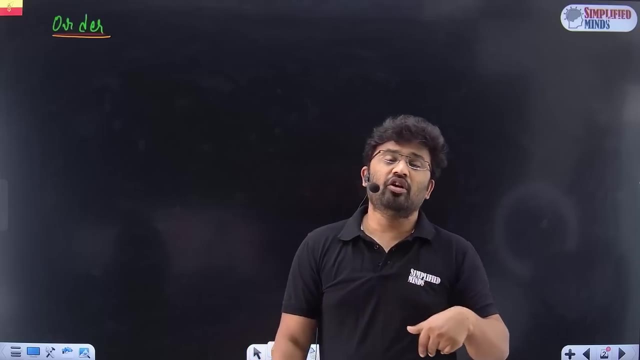 one function by saying order. You have, for example, here: here I have differentiated one side steadily, So sometimes we differentiate two times, sometimes three times. We have to eliminate that. So we learn that there is a separate topic. 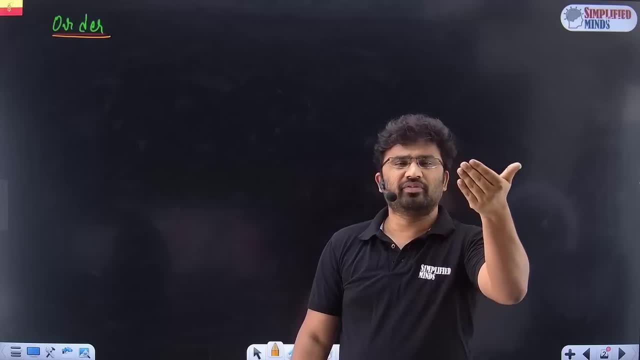 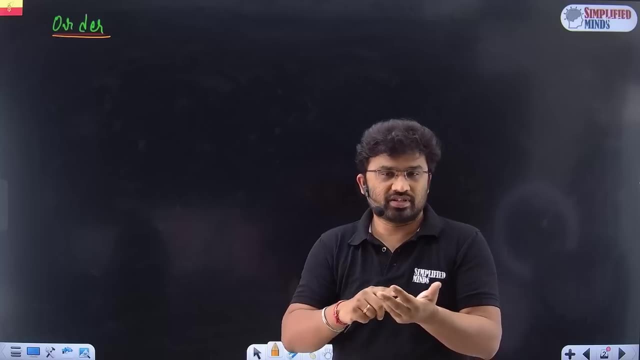 from the farming differential equation In that, how many arbitrary constants will you differentiate from that? But what I am saying is in order: how many times did you differentiate in any differential equations? First order derivatives. second order derivatives. third order derivatives. higher order derivatives In order. how many times did you differentiate in order? I will go simply. I will take an example: d cube y divided by dx. cube right 3 into 3y divided by dx plus our example 10 is equal to 0.. 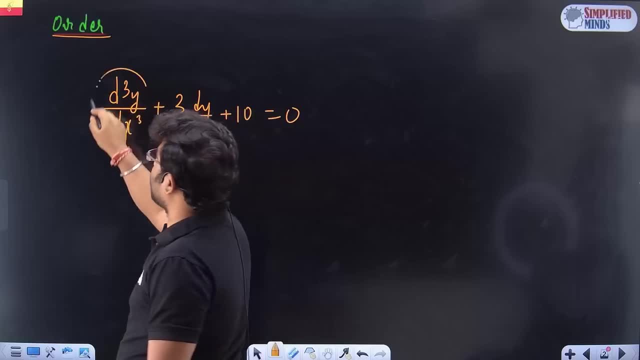 How many times did you differentiate? Highest differentiated? You have differentiated this equation three times Highest differentiated, So the order is 3.. So in order, there is no confusion. It is very, very simple, Very, very simple. 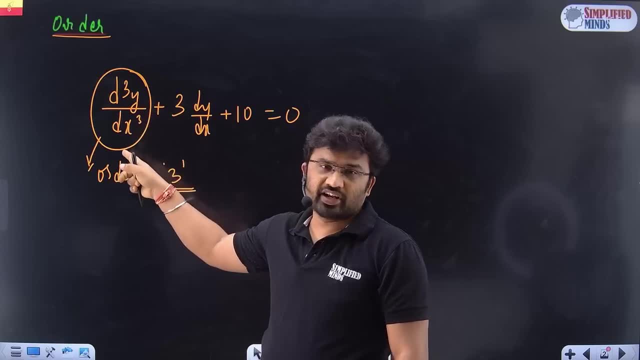 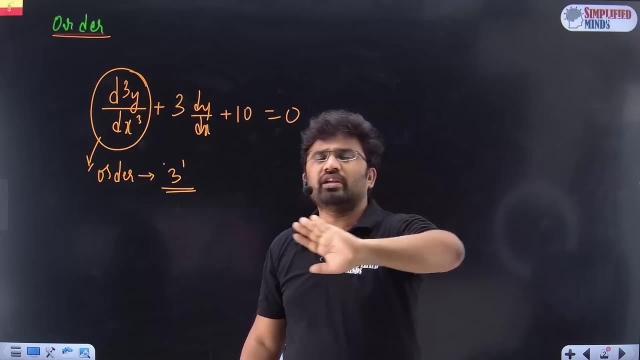 In any question. how many times did you differentiate? For example, this is differentiated one time. This is differentiated three times. So, in order, the order is the order of the equation. Simply So, the order has no condition. So in all cases, 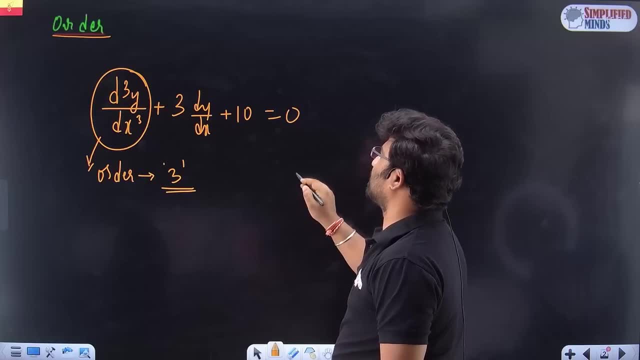 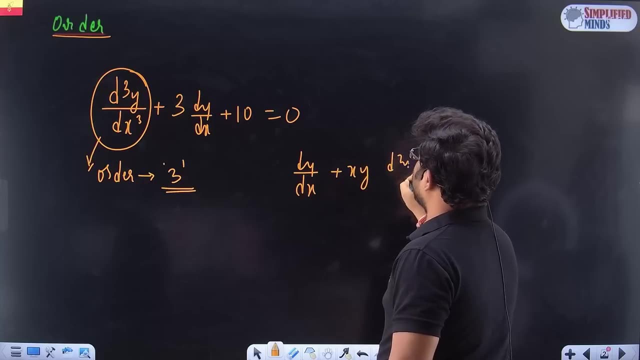 you can find the order easily, But there is something called as degree. There is nothing in order In any question. for example, in any question, you have d y by dx plus x y into. in any case you have d square. 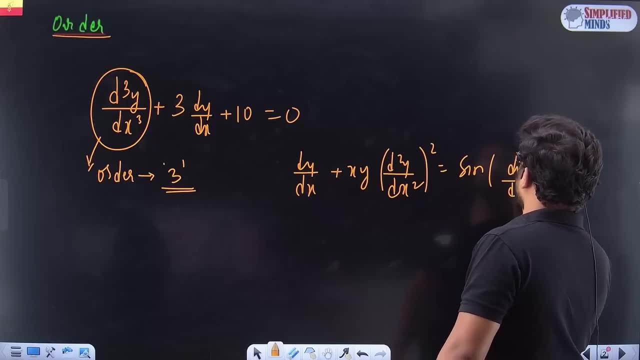 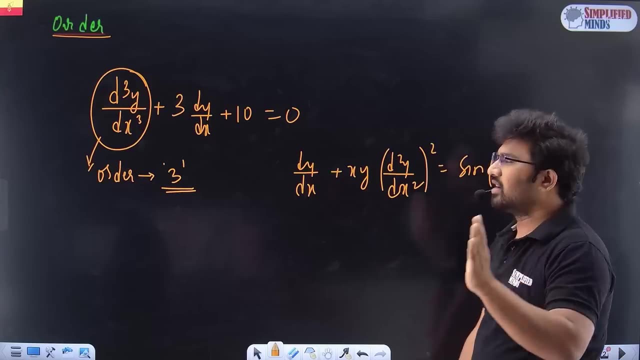 y by dx, square to the power of 2 and the sign of y by dx In any case. in any case, the highest test is 2 times. That is the order. So in order, how many times did you differentiate? 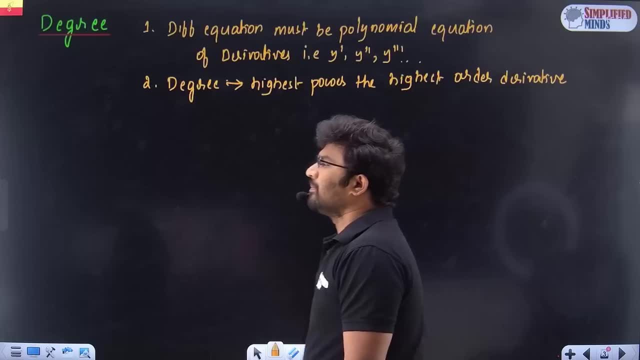 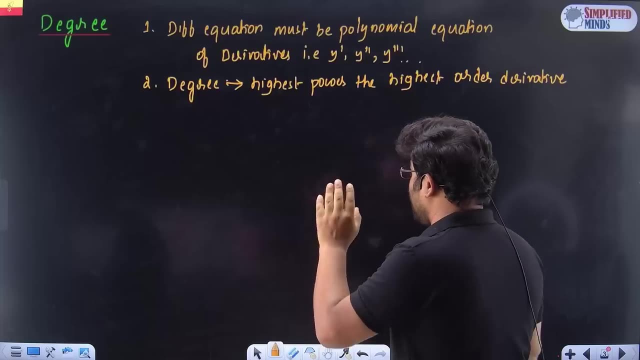 How many times did you differentiate? How many times did you differentiate the function Simple, So degree, What is degree? Basically, this is very, very simple. If you say degree, look, degree is very important. The degree defined by. 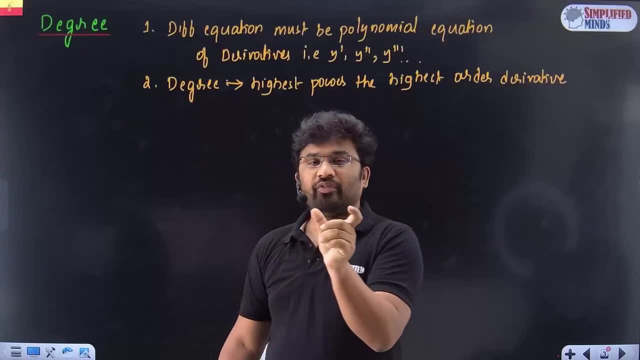 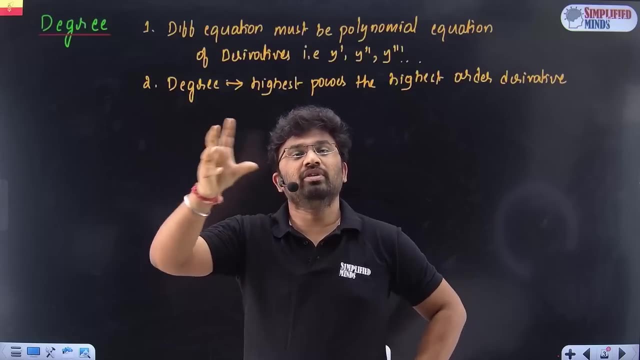 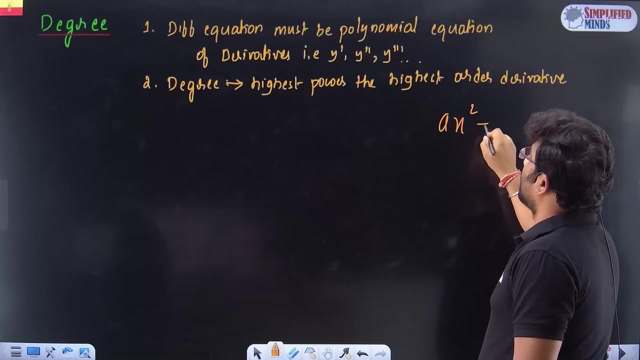 Kelvin is not defined by Kelvin. So now the first condition to find the degree is: whatever question you have asked, you must have the polynomial form. You know about polynomial right. Polynomial is basically so usually it's ax square. 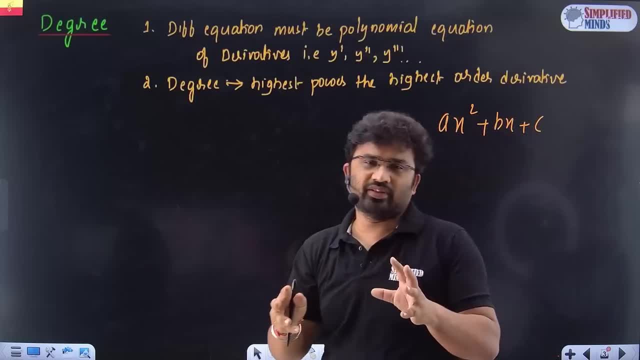 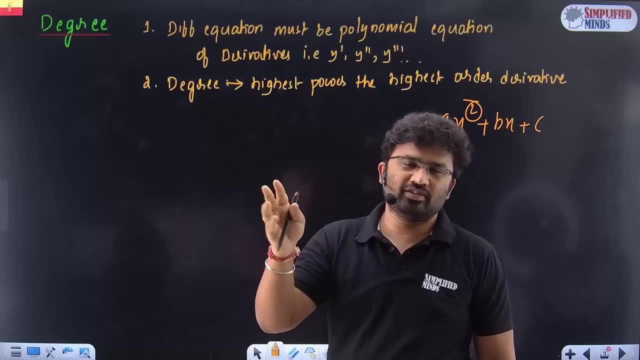 plus bx, plus c, where the terms are usually addition terms. Majorly there are exponents. right, These exponents must be whole numbers like 1,, 2,, 3,, 4,, of course, 0. Whole numbers are 0.. 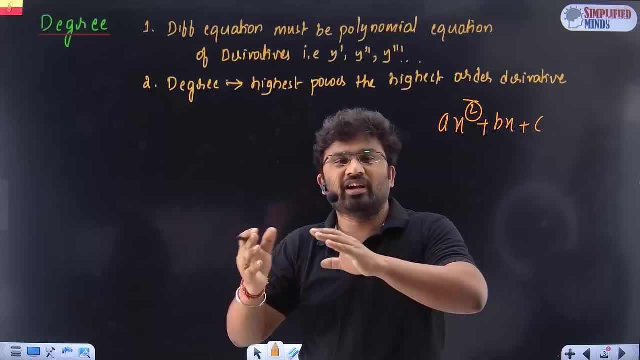 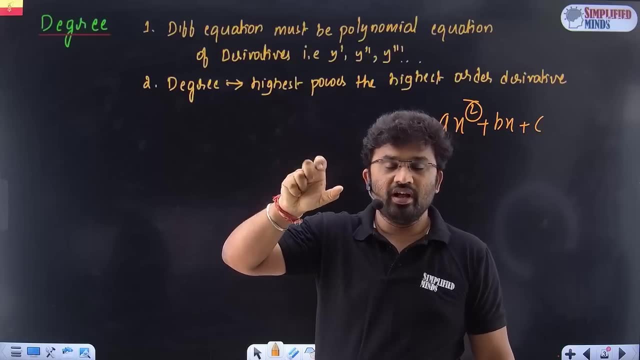 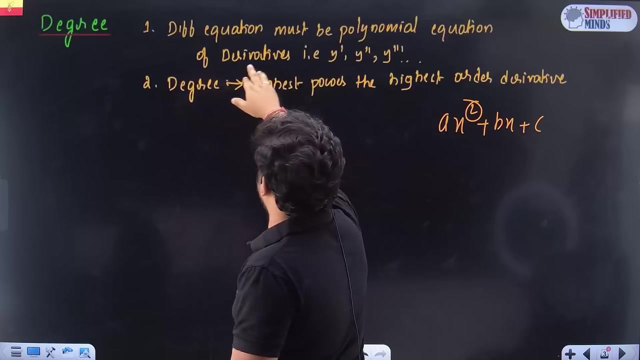 Natural numbers are positive integers only, So in polynomial form. So first of all, any differential equation should be in polynomial form, In the polynomial form of the textbook. the differential equation must be a polynomial equation of derivatives. So how can the polynomial equation of y, dash, y double, dash y triple 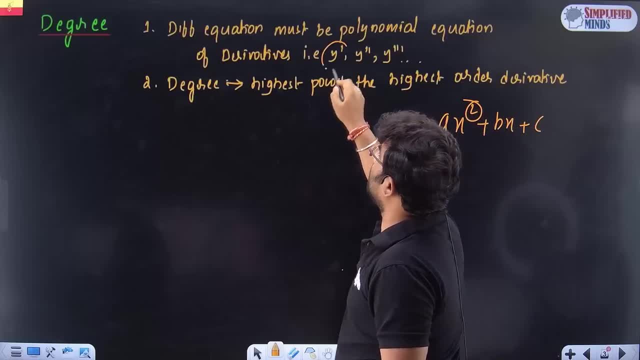 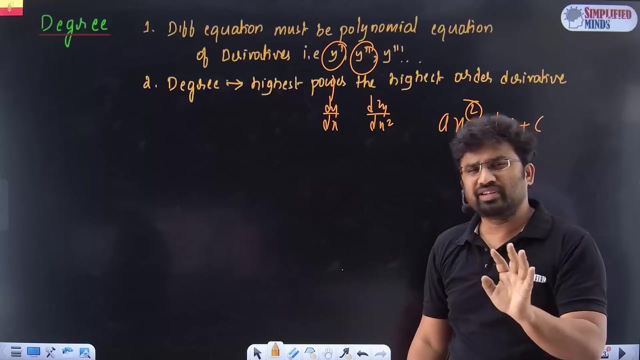 dash be. For example, y dash is basically another one. y dash is dy by dx. We use this formula everywhere in this chapter. y double dash means d square y by dx square y. triple dash means d cube y divided by dx cube. This is the general notation, Even in our first. 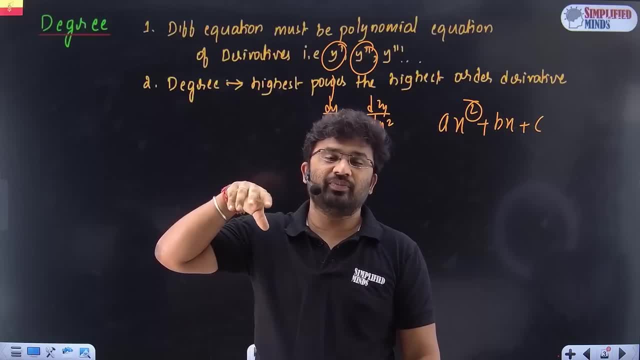 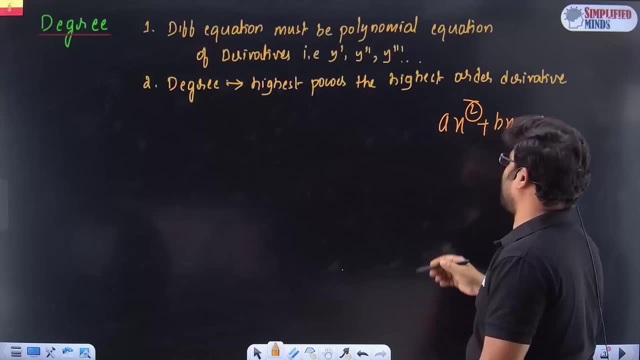 chapter. we know that higher order derivatives are a very important question. Higher order derivatives: We use y dash, y double dash there. Now, first of all, the polynomial formula should be: x into y dash plus y double dash, the whole square. This is the polynomial. 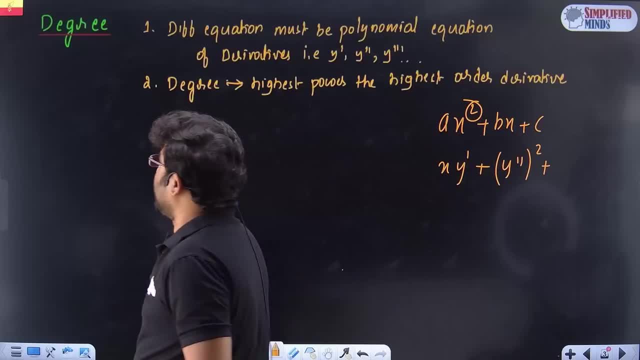 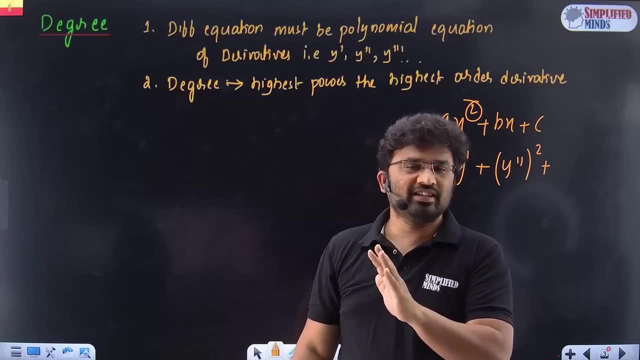 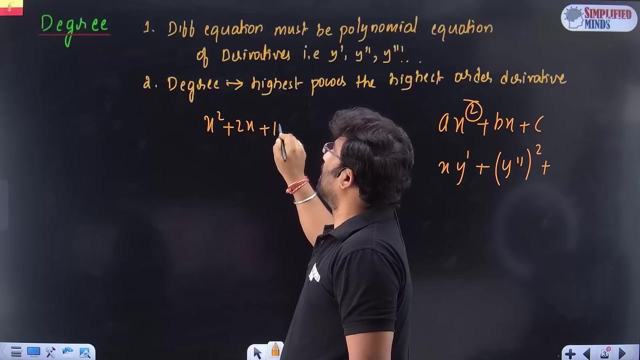 Now let us understand the polynomial. For example, if we take the polynomial functions of sin x, sin x, log x, we do not take the polynomial functions. For example, if we take x square plus x square plus 2x plus 10, if we take sin x, the whole square and then 2. 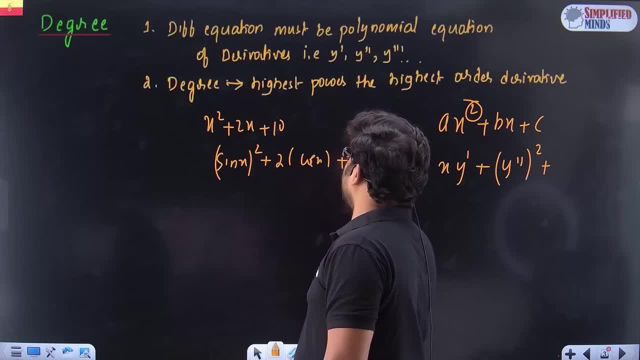 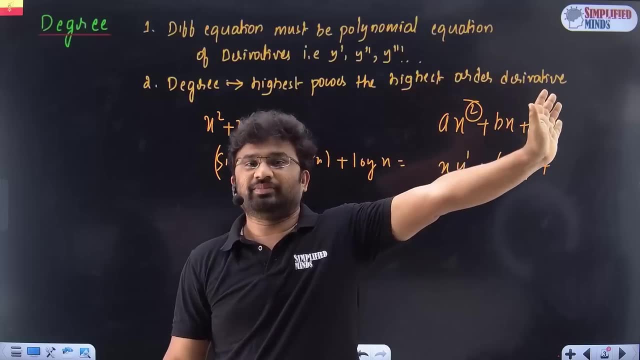 something like this: 2 into cos x, some log x, it is not a polynomial function. It is not a polynomial If we take the polynomial functions of sin x, sin x, log x, exponential functions. if they are like this, we already know that they are not polynomial functions. So I can tell. 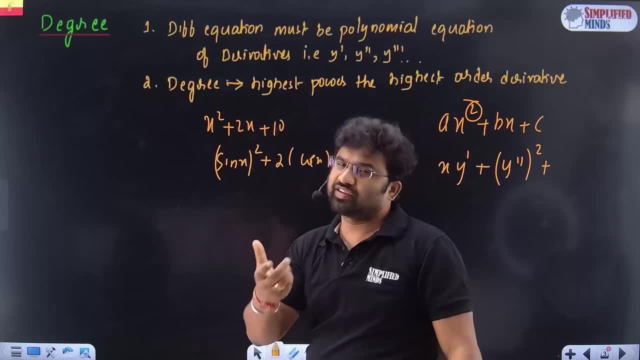 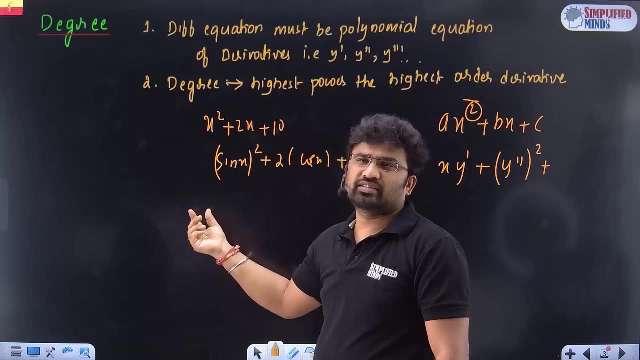 the reason also. Actually see, basically there is an expansion for sin x, For example. if you take sin x you will get something like Taylor series. If you use that, you can expand sin x, x minus x cube by 3 factorial plus x to the power of 5 by 5 factorial. That. 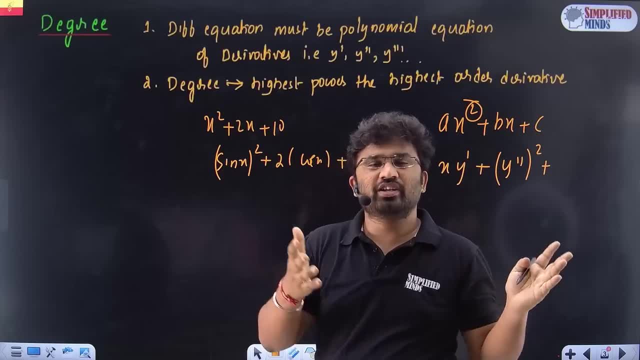 is the expansion. It is in series and sequence. So there is an expansion for sin x and log x, In that you will know the higher standard In the higher standard- Sine x, sin x, log x- you will also get the polynomial functions. So that is why some 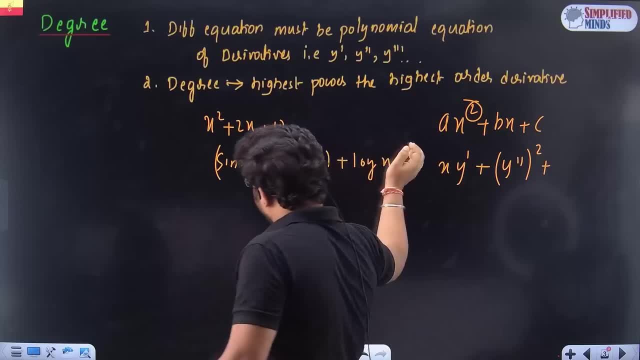 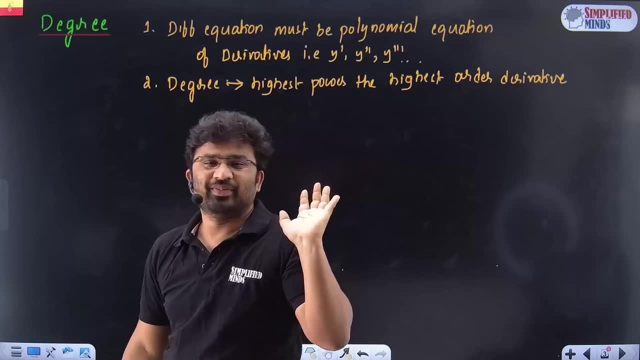 times degree is not defined. Maybe this will not be the case. if you understand what I told you, I will take the questions. See, do you know what is Maths In math? you cannot understand how many words we have in math. How many words do you have to say in math? Maths doesn't. 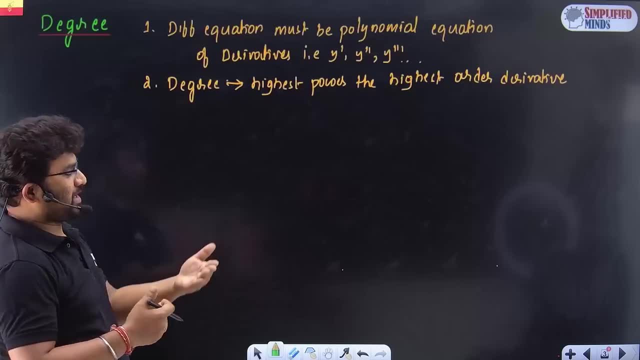 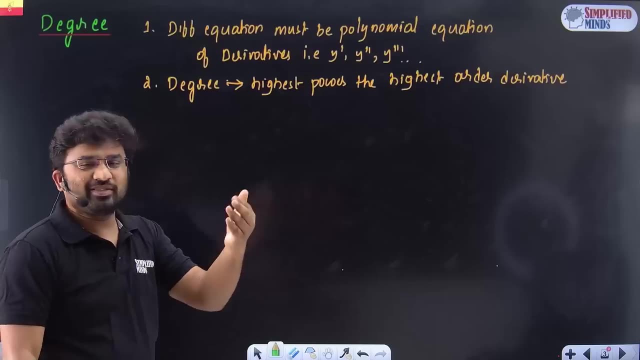 go in the head. It goes only when you ask questions. Maths can never be read. That is why I said You can't study maths. You can study physics, chemistry. you can read and understand Practice maths. until and unless you keep the pen on the book, you will never learn mathematics. 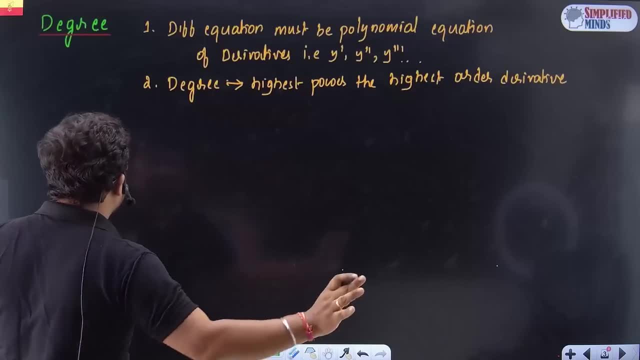 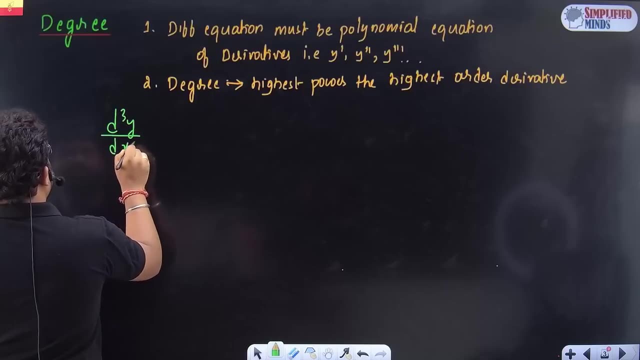 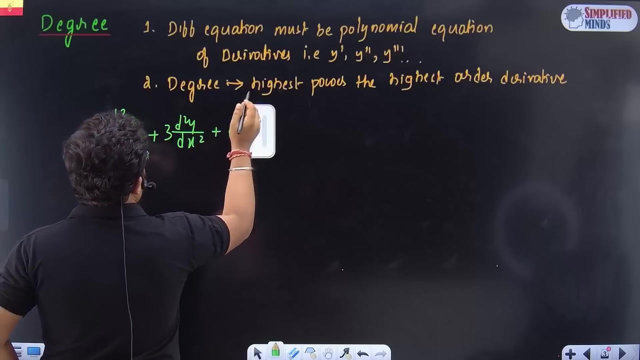 Anyway, I have said something. If you don't understand, it's okay. I will take some examples. first Let's take some random examples: D cube y divided by dx cube plus. let's take 3 into dy divided by dx. Let's take something called 3 into d square y by dx square plus. 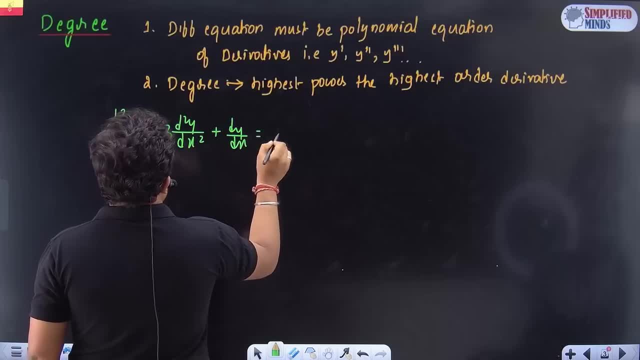 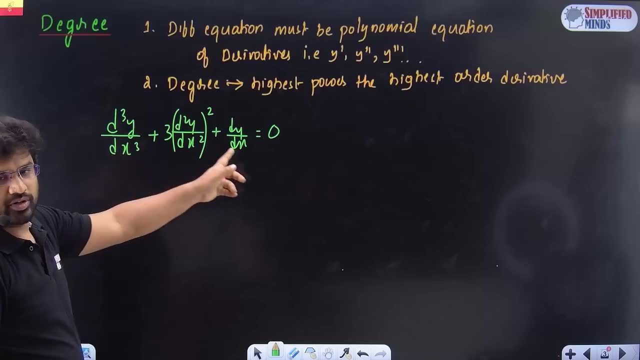 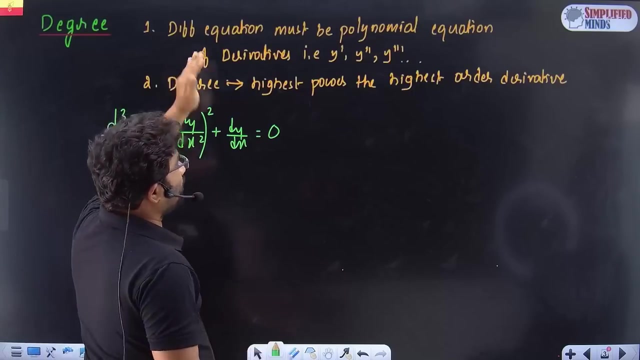 maybe dy divided by dx, That must be equal to 0.. Simple example, For example, this is square. So clearly, what is the order of the equation? Order is very simple. The highest time differential is the order Degree. So if you want to define the degree, degree is the highest power of the highest order. 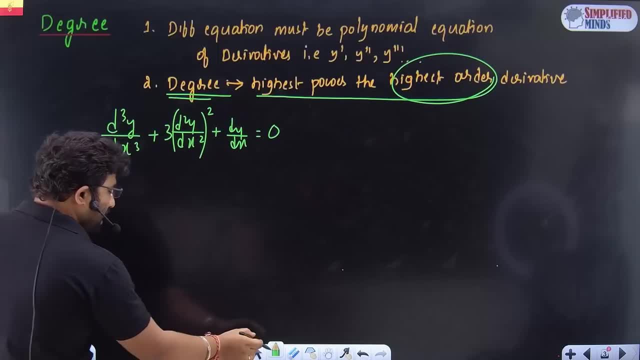 What is the highest order? Can you use the highest order? Can you use the highest order? This is the power of this. Some students get confused. I have said that the order is the highest of this. You both snacked on the ninth, So there is no order here, But there. 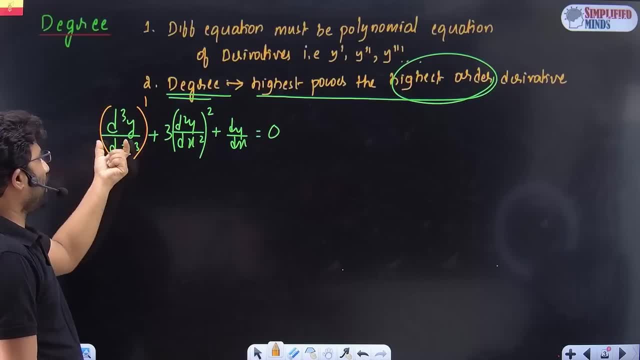 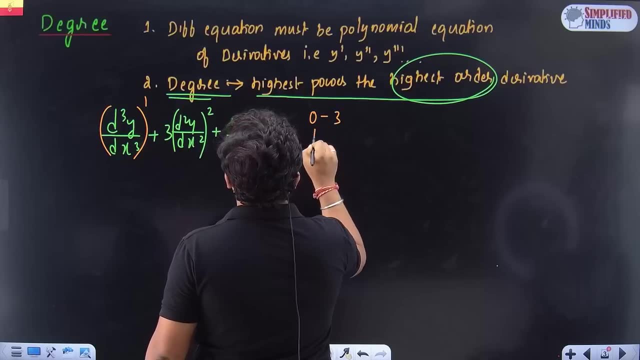 is degree. This is the power of this. What is the highest order? So, for this question, what will be the order? The order will be 3 and the degree will be 1.. Is that clear, Simple? These are straightforward questions. 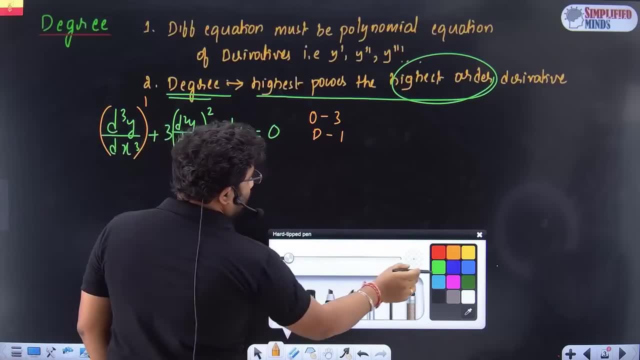 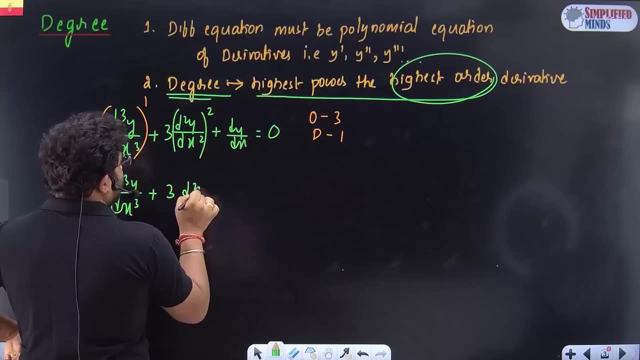 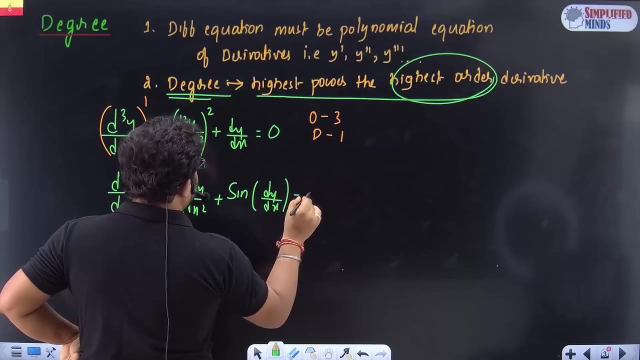 So one way. I have one question, For example. I will take one more question now. The question is: d cube y divided by dx, cube plus 3, into d square y by dx square plus sin of sin of d y by dx. So what will happen now? The sin function is coming inside y, So it is. 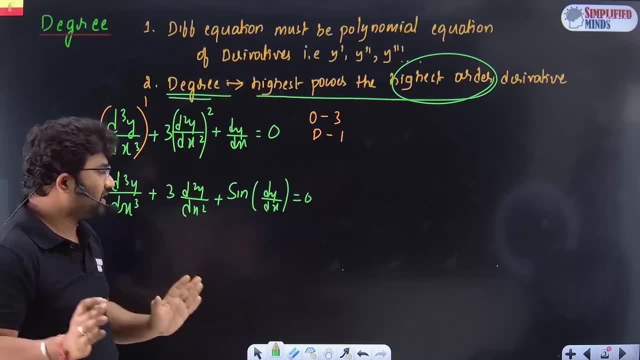 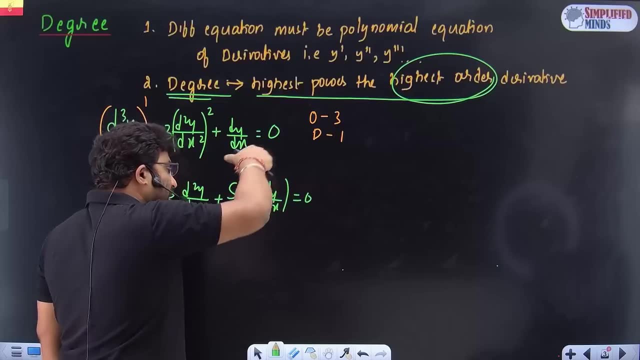 not as per. it is a polynomials of y dash. So, in any case, look at sin of d? y by dx, or cos of d y by dx, or log of inside d y by dx, or tan of d y by dx, or e power d y by. 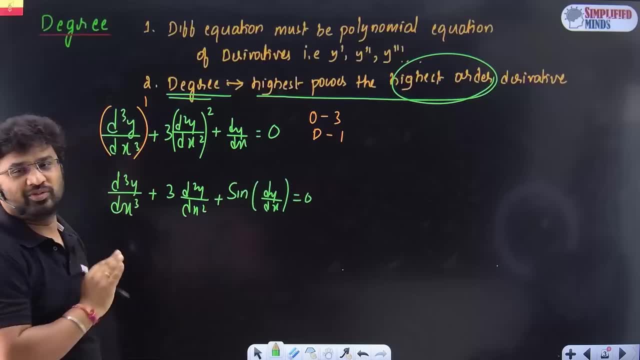 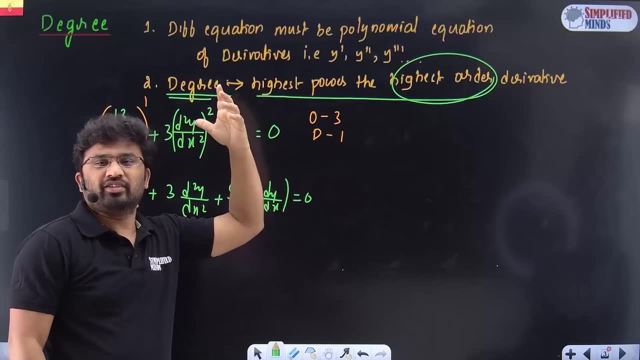 dx. So if there is another function, it will not become a polynomial. So in that case, in that case, because, as I said, sin is the expansion, Cos is the expansion In that powers will come. So we cannot tell exactly. So for 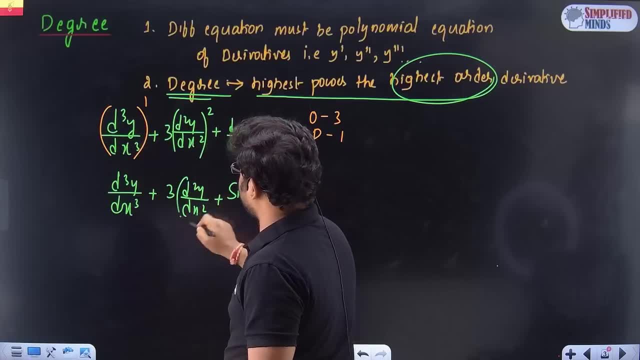 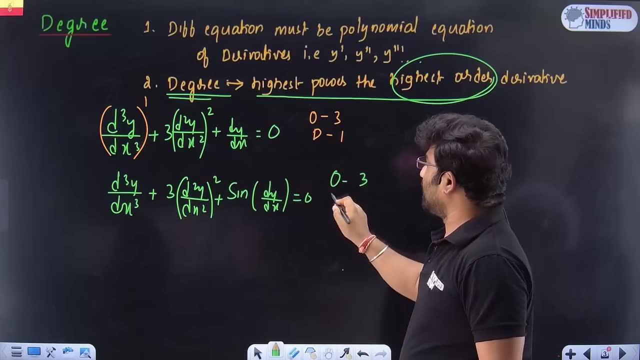 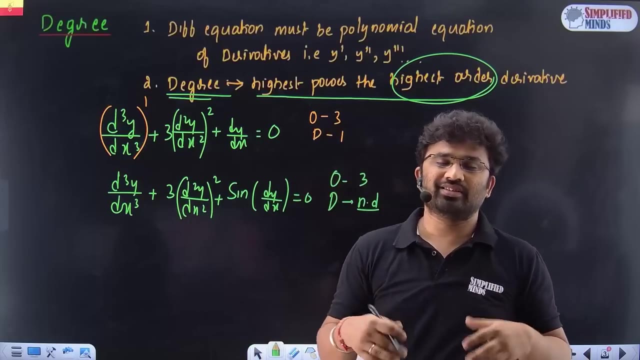 this we can clearly say, if we take really square: the order is defined, So the order is defined. The degree is not defined, So whose degree is not defined Whenever there is a sin, any function, sin, cos, tan, e, power, any mathematical function inverse. 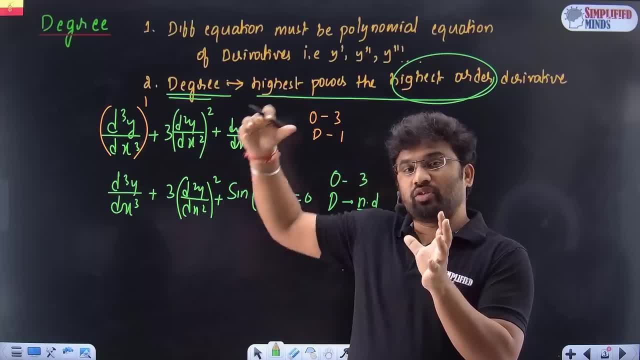 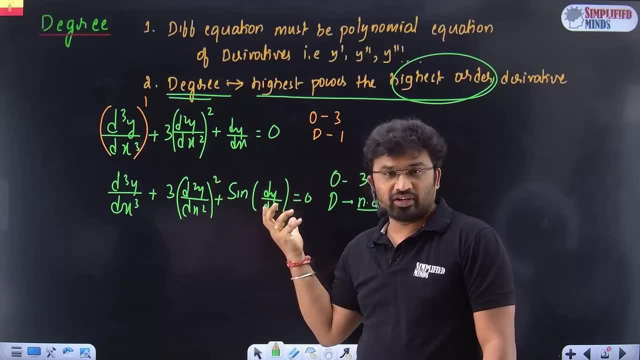 trigonometric function, log function, tan functions, that function will have another y dash inside y dash. The error cannot be separated, right? You cannot take it out, So we cannot modify any thing or do anything. In such cases, degree is not defined. I will. 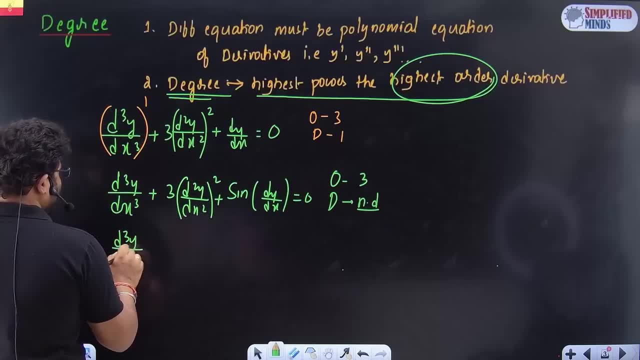 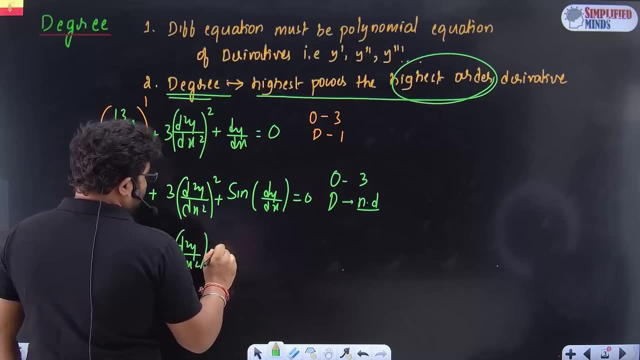 give one more example. So we will do some more examples Now. d cube y. I will take this question. I will modify this question d square by dx square. Here we have sine y. The sin y is equal to zero. See, if you see this, it is normal In this equation. 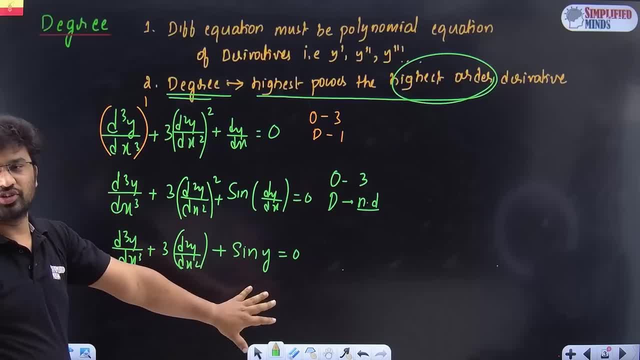 the sin y is going to be 0. But in this equation if we take the downside of y dash, we cannot take out this small negative. So, for example, if we take y dash we cannot take out. It is definitely a polynomial function. 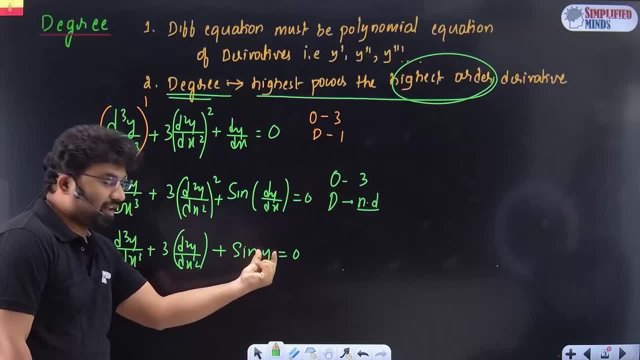 Here there is y triple dash and y double dash. Inside the sine there is no y dash, y double dash or y triple dash. It is just a normal sine, y function. In both the order is defined and the degree is also defined. 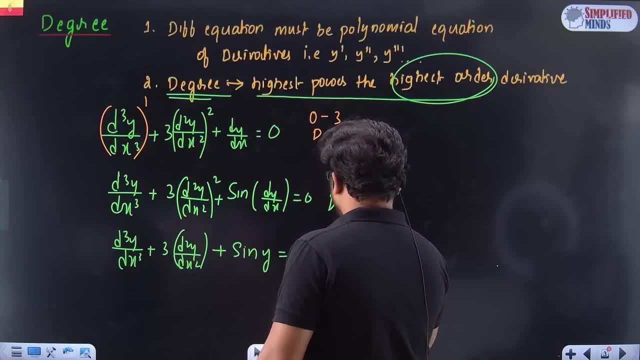 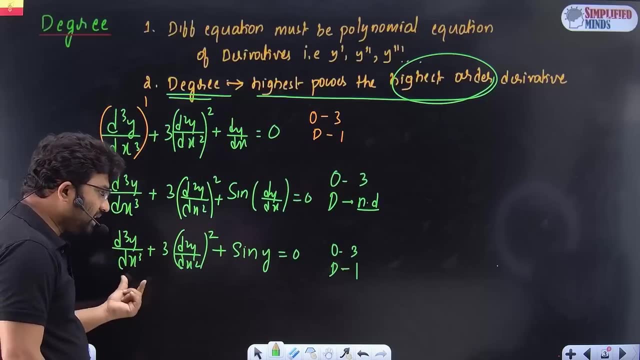 So the order is 3 and the degree is obviously 1.. Because this is the power thwomic, This is the power thwomic 1.. So the order is defined and the degree is defined. Understand this: The function of sine cos tan, etc. 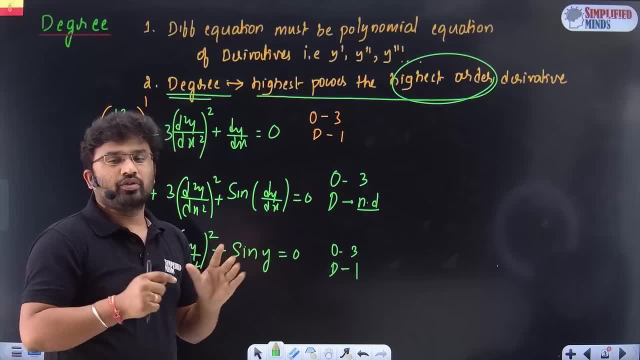 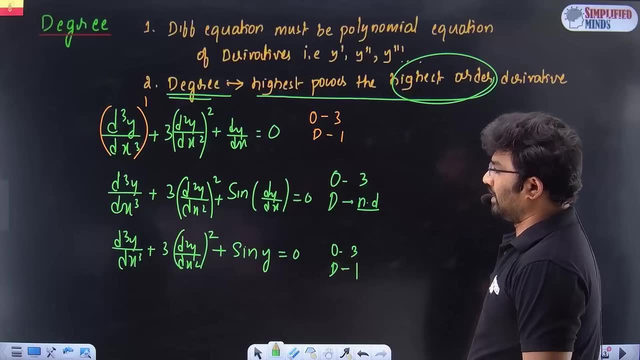 Inside that y dash, y double dash, y, triple dash, etc. are not usually defined, But there are some cases where we can do this, For example- I will give you a simple example, For example, sine inverse of, or I will say sine of. 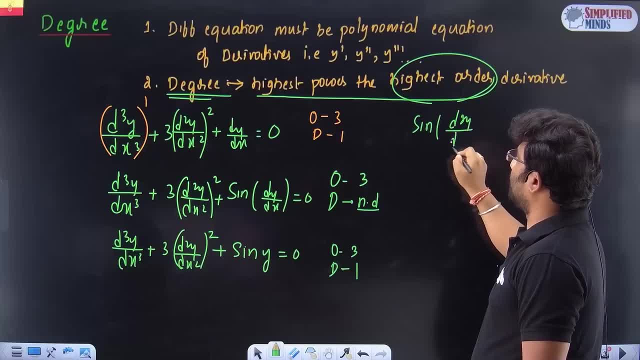 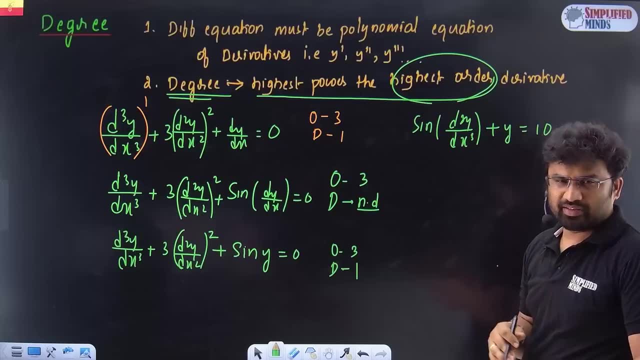 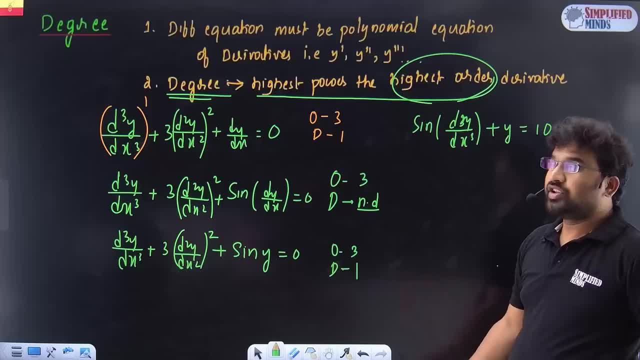 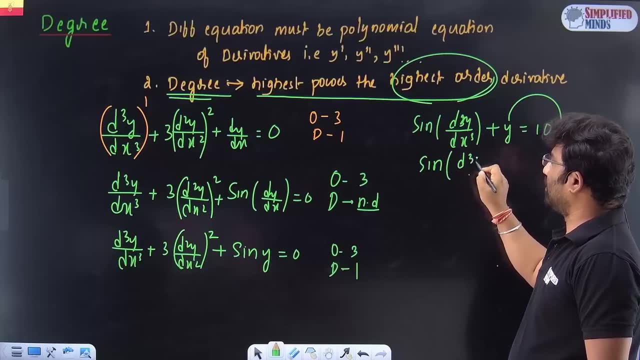 Similarly, you can see the inside of sine and cos. You can try to simplify this, guys. To simplify, I will shift the y Sine of d cube y divided by dx cube 10 minus y. You can shift y because you want the sine. 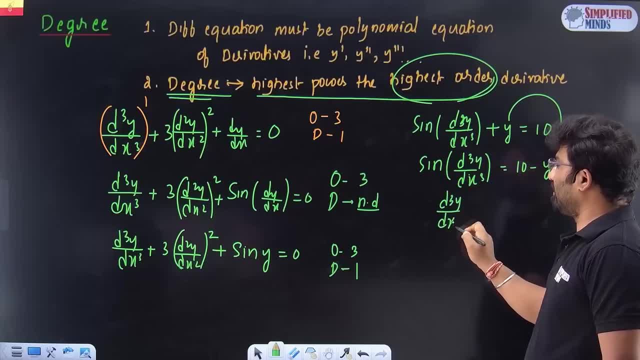 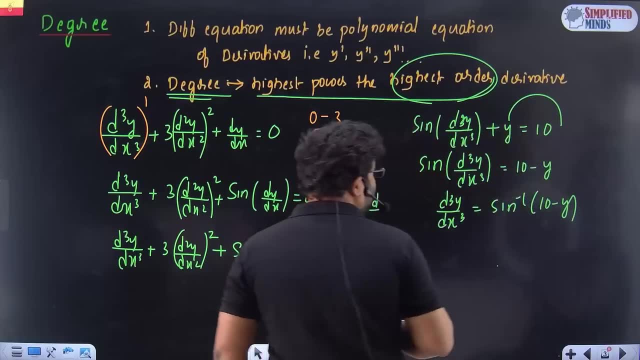 When I shift I get completely d cube y divided by dx cube. Here I have sin inverse of 10 minus y, Or I can shift it to something else. I can clearly get it. I got eliminated. This sin is here right. 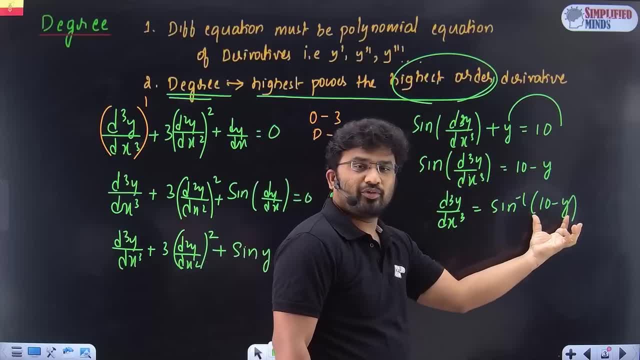 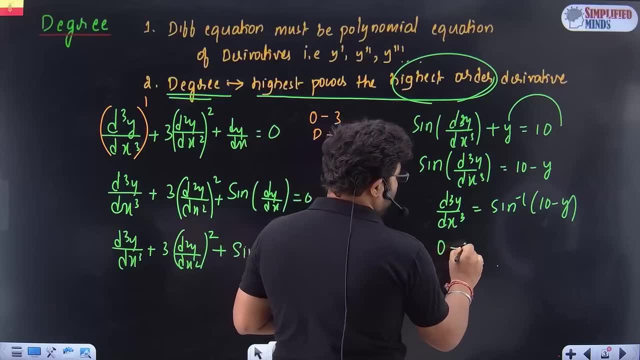 I shifted it there. When I shifted there, there is no y dash or y double dash anywhere, So there is an order degree for this. What is the order for this? Simple, The order is 3.. The order is 3.. 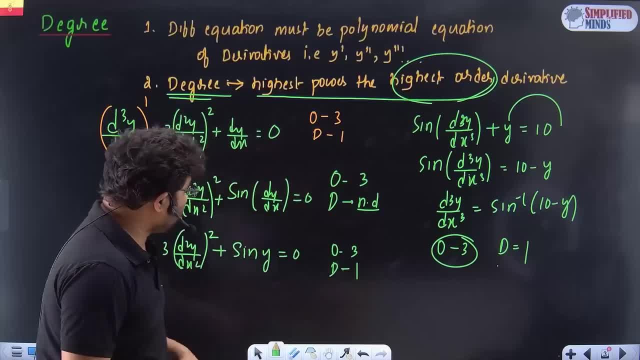 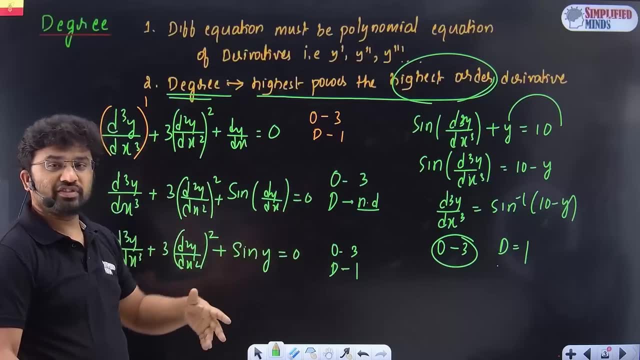 The degree is 1.. But, sir, how can I do this? How can I do this? There is sin of d, y by dx. I shift it there, I shift sin there, Sin inverse of 10.. Inside that, y, double, y, triple, dash, y, dash will come. 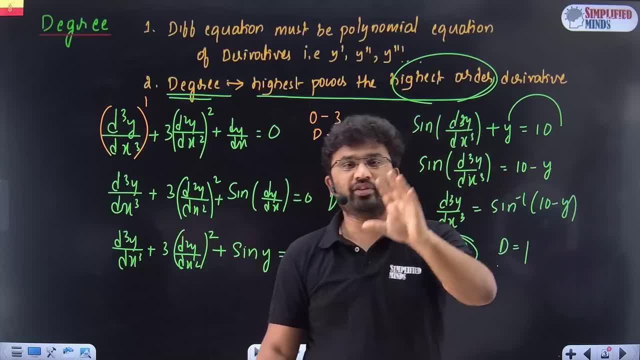 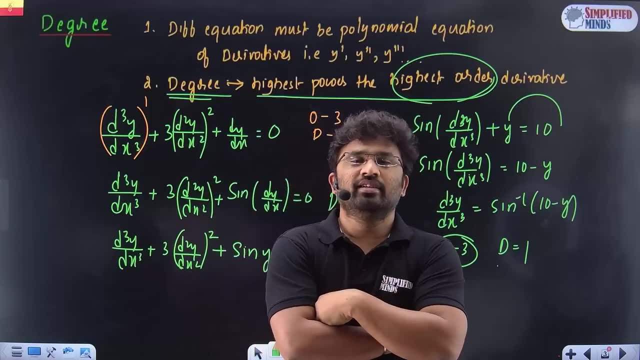 See, you should not have So inside sin cos log. whatever is there inside that function, there should not be any y dash or y double dash. If there is none, that is called as. If there is none, it is defined. 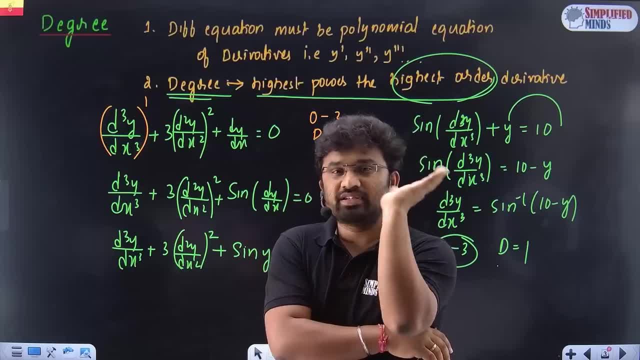 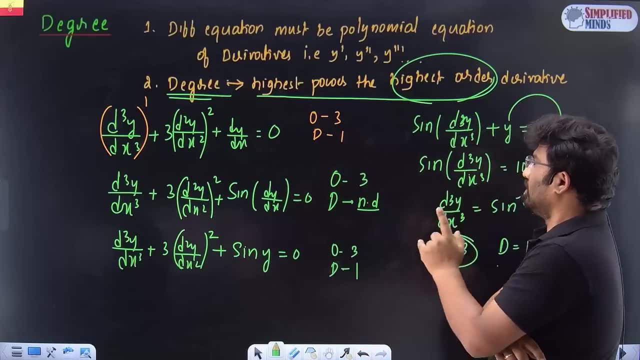 If there is none, the degree is not defined. Order is always defined. Order is very easy. If there is none, the degree is not defined. Is it clear? Is it very clear? I hope it is very clear. This question is asked in a lot of exams. 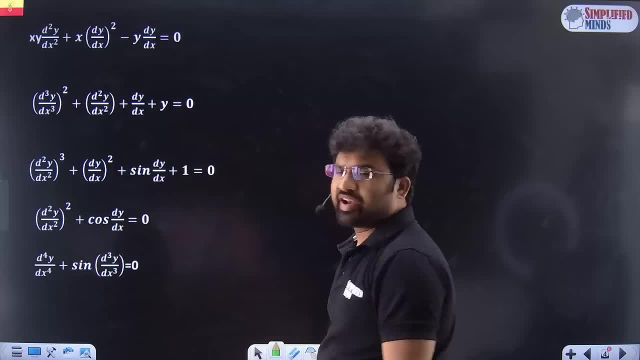 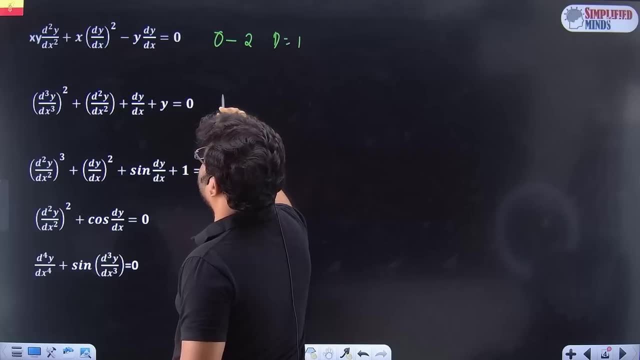 After that you can find the order degree for all these questions. So what is the order degree? So the order for this is 2.. The degree is 1.. The order is O and B. The order for this is 3.. 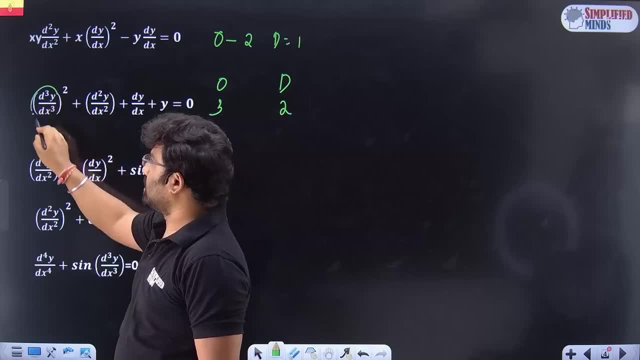 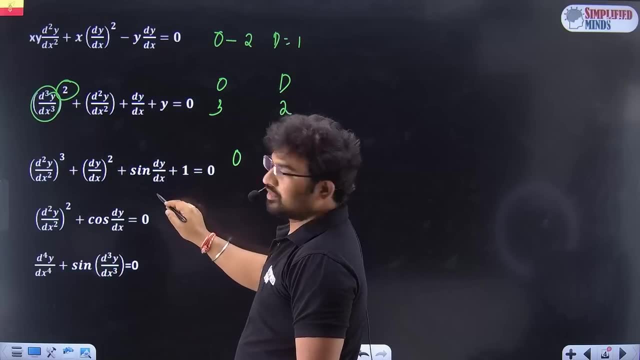 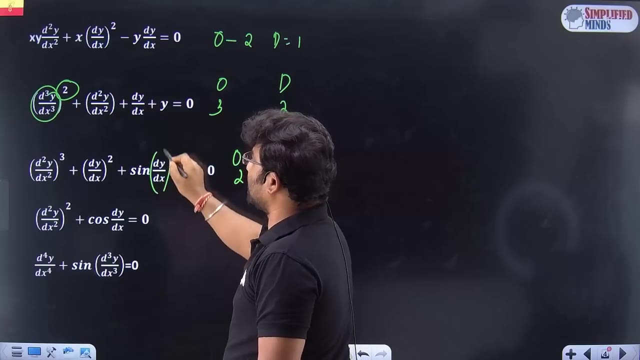 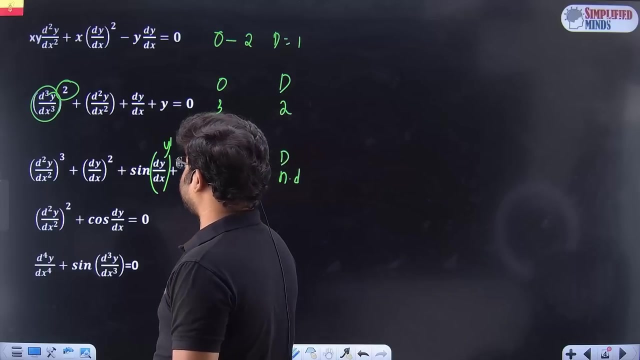 The degree is 2.. What is the degree? What is the highest order? The order is 2.. What is the highest order? The ordered for this is non-defined. What is the order for that? What is the order of this? 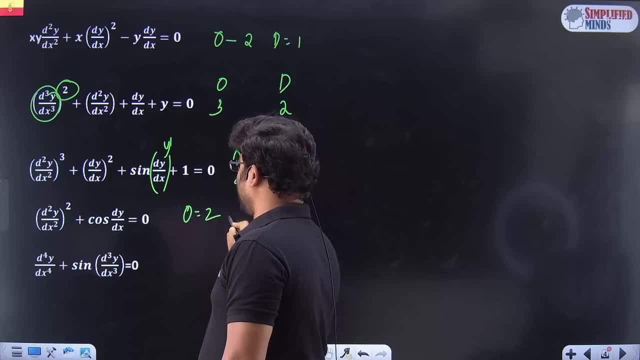 How to get the y dash. Here is the order, though not defined. yeah, can cause already function in there. they did d power 4 by d4. it was there. you do define. I give it a lot. I would like in there a new, new hell. what's an unique, a shift, more with Allah. that means I need to 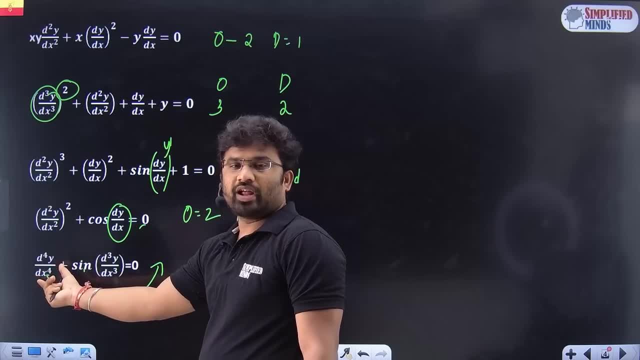 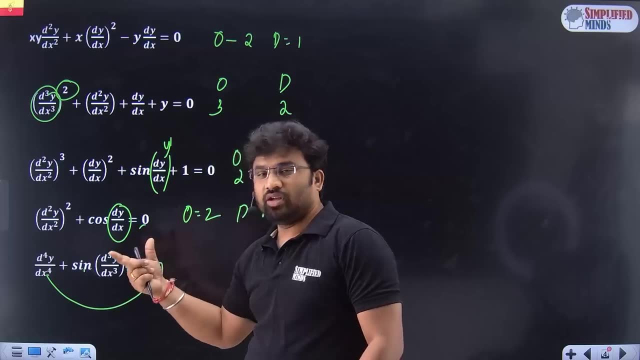 convert any, you will get the sin inverse of white, white for dash. why d4, d4, y by D, D, extra power for a glue define. I go to the lab you shift tomorrow. no, a sin cause for everybody why you're back on that kind of number, so constant, so why? 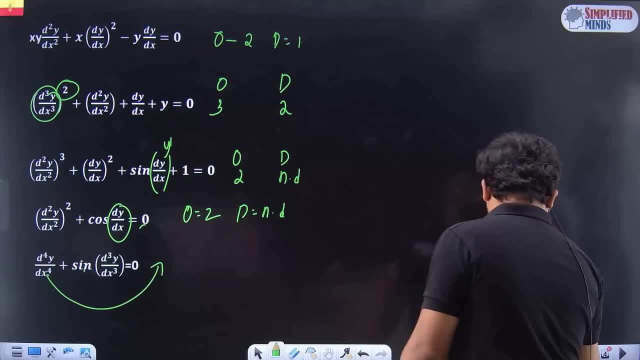 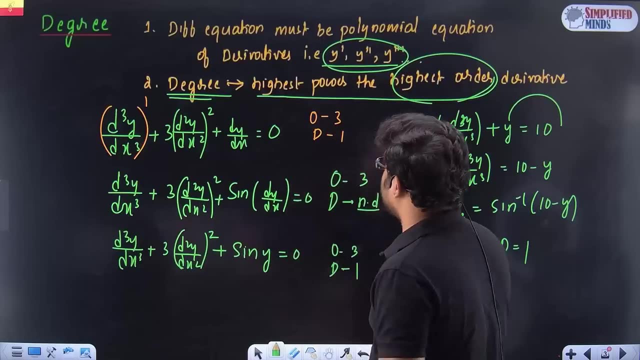 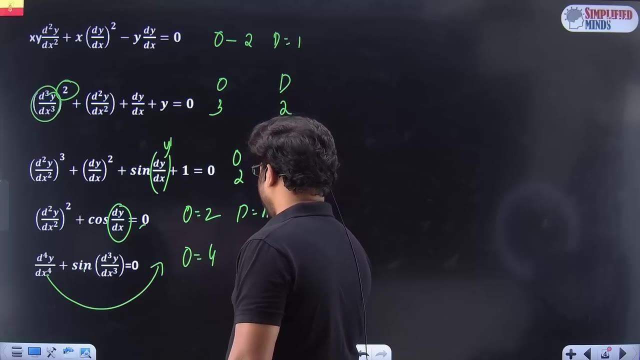 enter back why you dash, oh, why double-dash, why triple-dash is bar. do really clear, I healthy willy. so it should be a derivative soft. it should be polynomial function having derivatives of y, dash, y, double dash, y, triple dash, unity. so you do a step a harder than the order. when the four is: oh, degree bundle. 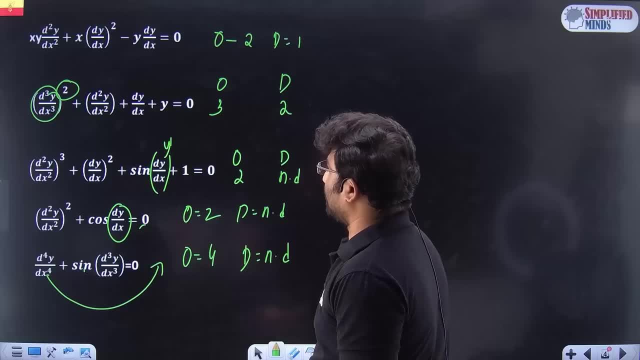 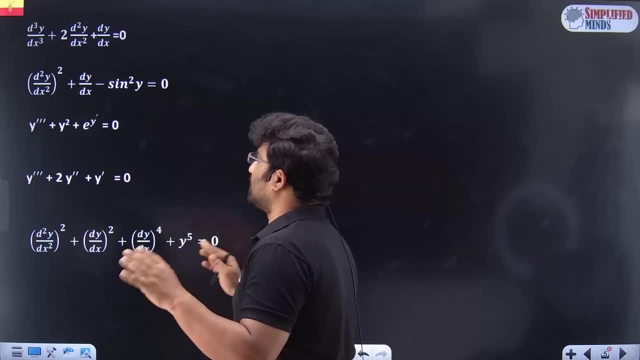 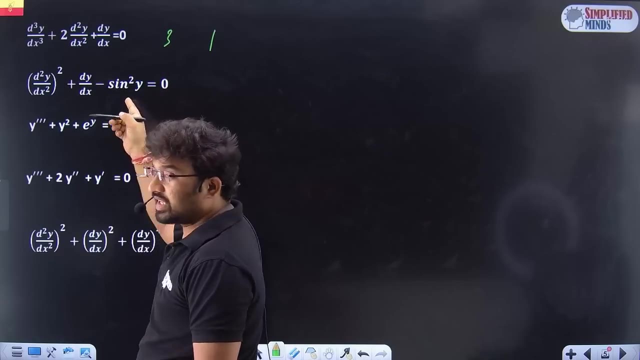 not defined right now. not define about that. okay, are that clear again so that my next two, next question window again even your video possible in your money, okay. so what is the order for this? you three degree degree one to one order for this order defined, I did it. 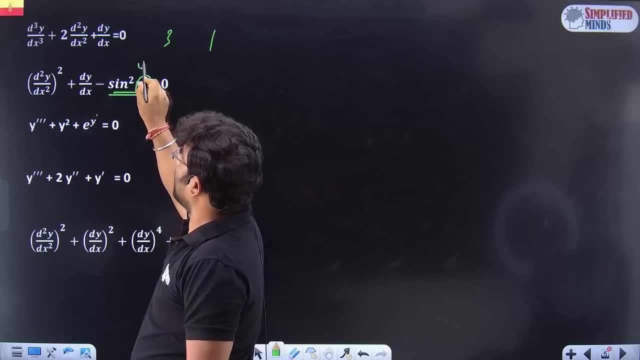 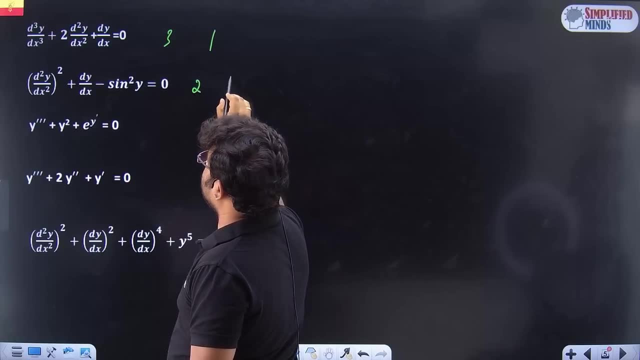 authentically sign in the L while you do all the other, the other, the other, y dash, y, double-dash, Hilda, and the course could order degree error to define Agatha, the order one, this to two degree, one though other the power to know, didn't know what is this now, why triple-dash? and they dq y by dx cube y. 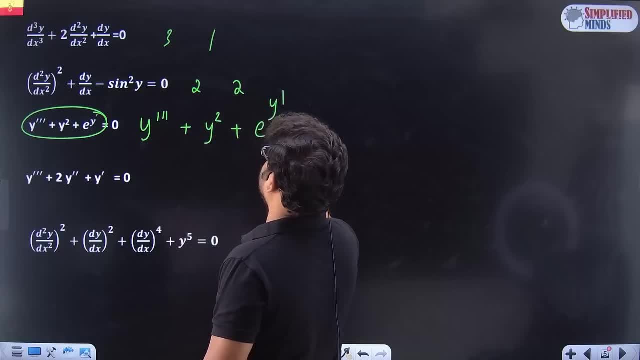 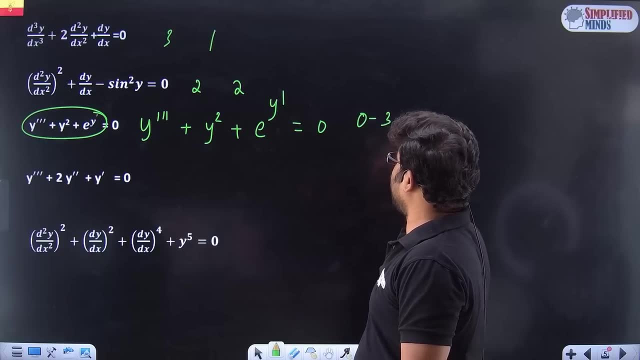 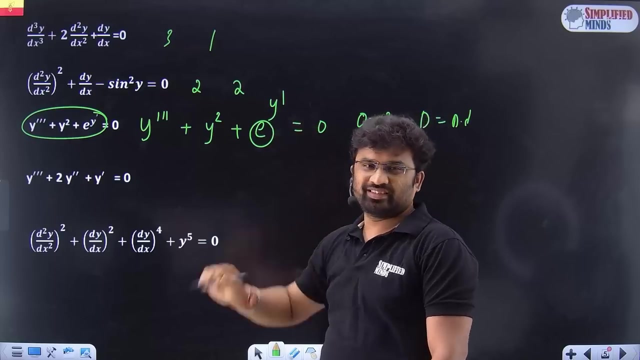 square with a, but the e power y dash it a and the Reno e power dy by dx, by dx, definitely so it. do you really going to order order when they know, maximum of the three degree, when the degree, when the not defining anything not defined, oh, now the exponential functionally other, on Billy Y dashes are: 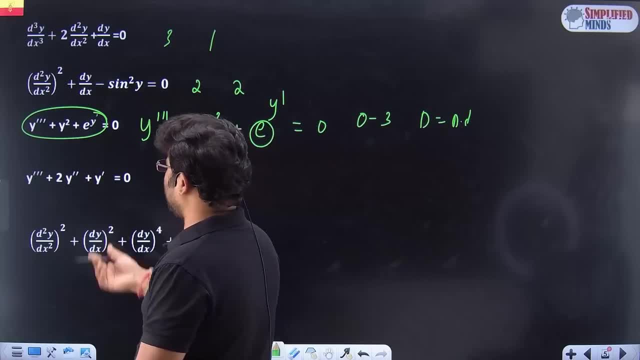 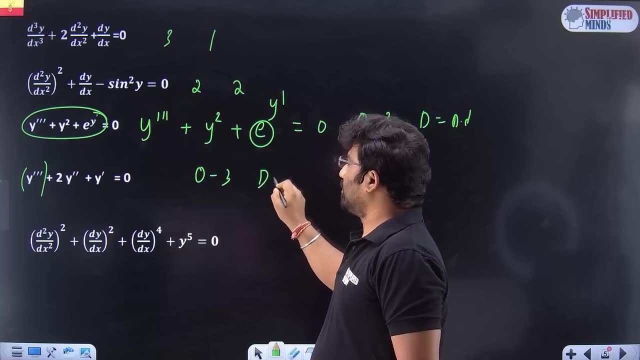 slightly again. give it a next-up, a white triple dash to a the define. I give them a why triple-dash in the e cube, y by dx cube. so order bundle three degree, bundle 1: right now. that made Esquire by dx square. okay, same thing we do, even you are. 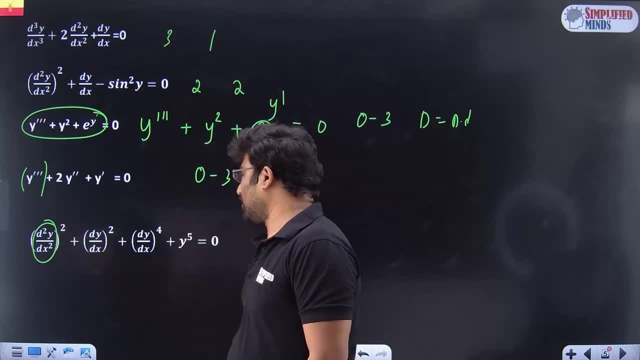 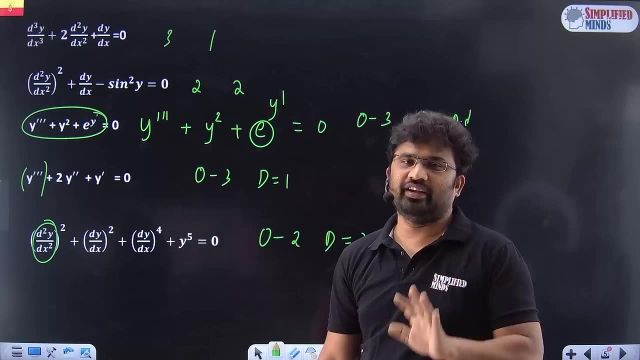 So what is the order is? ist is d square, y by dx square. that is, order is 2, degree is 2.. Is that clear? So that is all about order and degree. Now, if you understand order and degree, let us go for next question, next topic now. 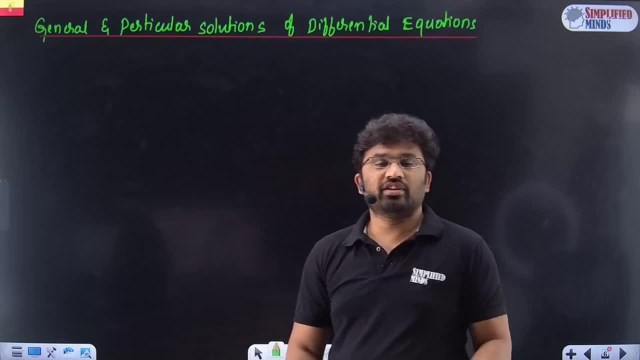 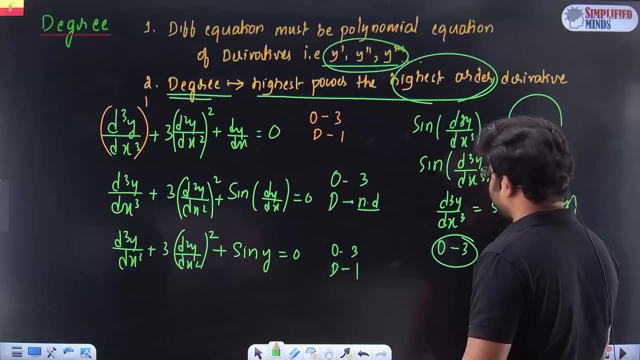 General and particular solutions of differential equations. So what is general solution? What is particular solution? I will give you a simple example. I will give you a simple example Now, starting with an equation. it is like a simple question: What is it? 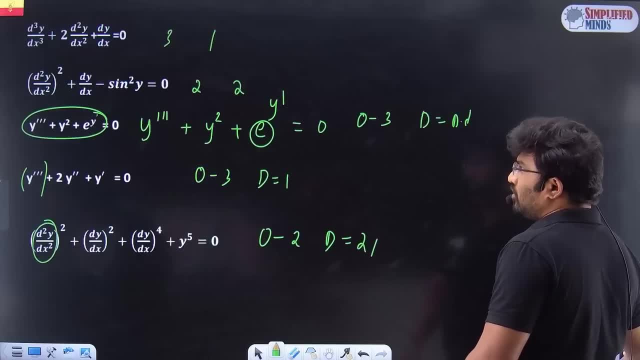 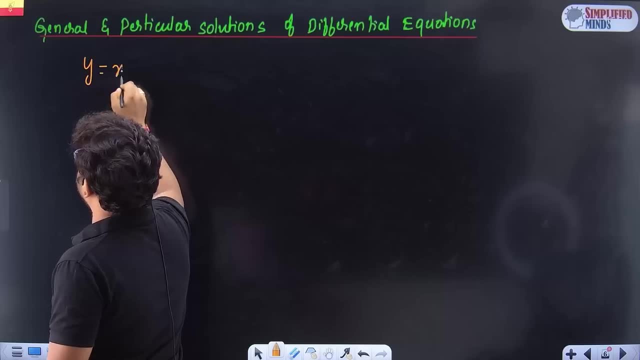 It is: y is equal to x square plus 2.. I will ask the same question, For example. I will ask a simple question. I will ask: y is equal to x square plus 2, x square plus a. I will ask: y is equal to x square plus a. 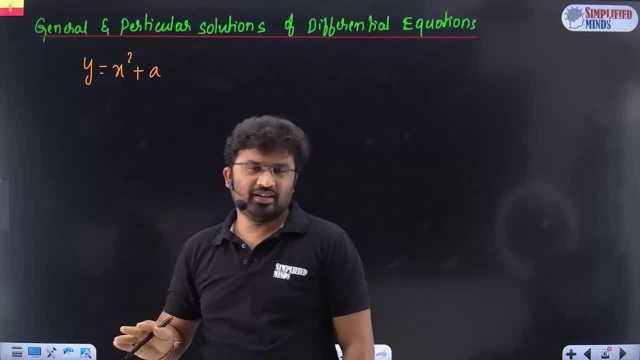 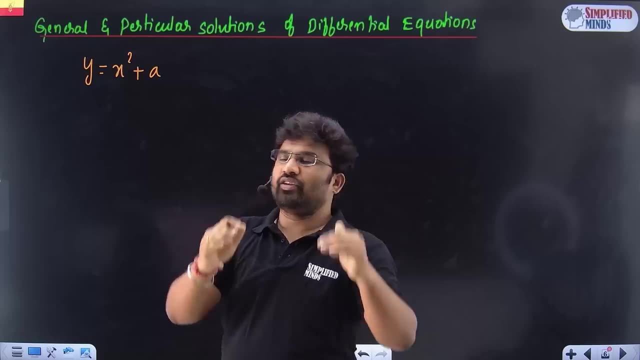 So you will get. basically it is like a family of parabolas: A1, you will get some. A1, you will get one curve. A2, you will get another curve. A3, you will get another curve Like this: y is equal to x square plus 2.. 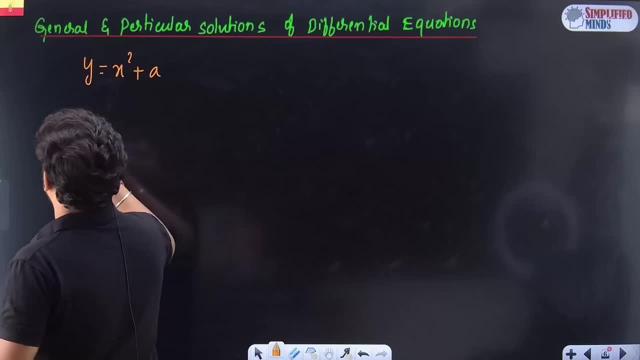 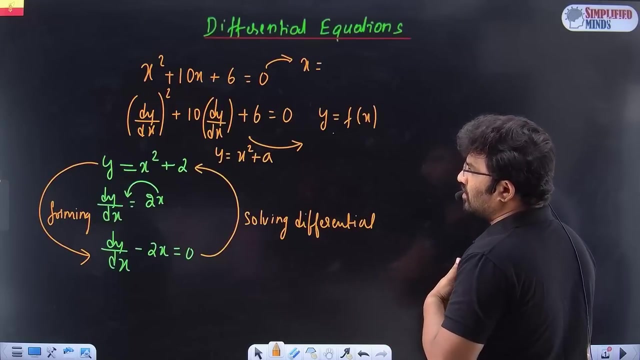 say: i know, though it is solution and differentiate matter. you know what the basically so in differentiate what you're going to get it. so, for example, uh, i'll take reverse way and in the reverse i'll quote one name: share, uh, what the question is. we got dy by. dx is equal to x alpha. 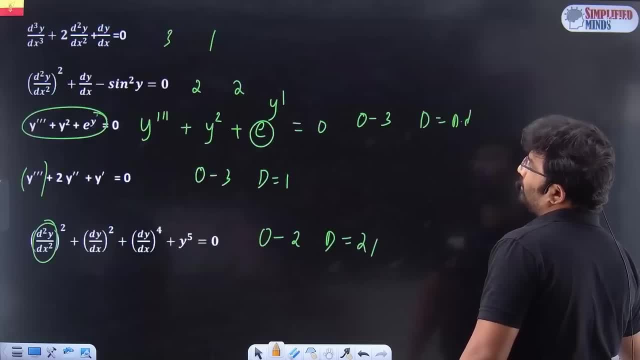 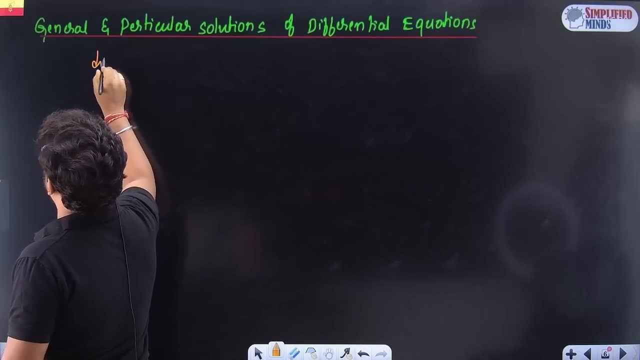 dy by minus dy by dx minus 2x equals zero. okay. other question, just simply explain, okay, uh, sorry. so let's take a next differential equation: d? y by d y minus 2x, equal to 0.. this is solution. find body and character. as i've told you, we have a separate lecture again. 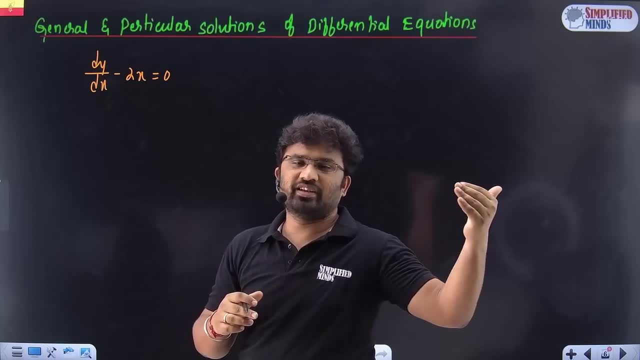 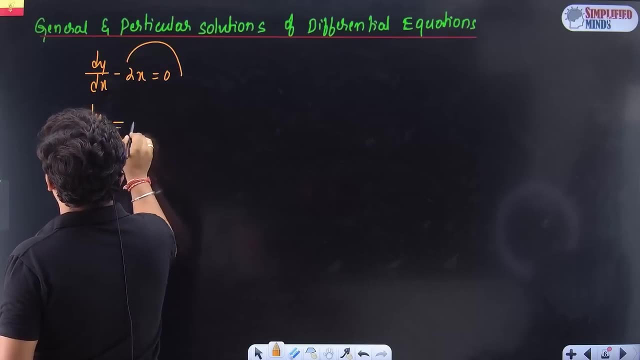 solution method: okay, different, different methods, linear, homogeneous, linear variable, separable under, but really simple health code in the solution. find one. i'm going to do it by dx, because you should equal, shift out 2x. i'm going to shift the dx this side, so dy is equal to 2x into. 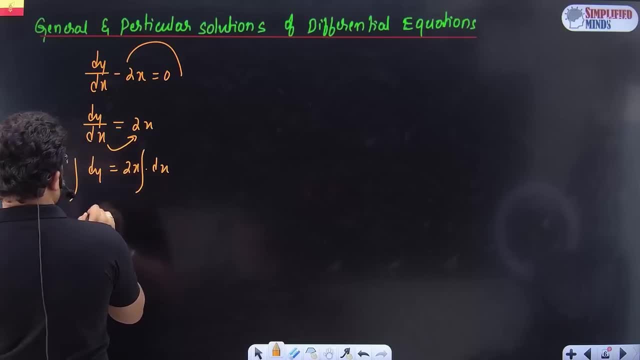 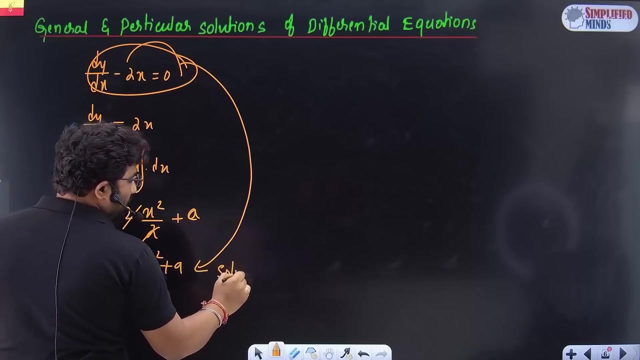 dx. that means x squared by 2 plus c plus constant, or some value plus a, some some value should be there. so 2, 2 cancel over the y is equal to x square plus a. so e differential equation: yeah, in the solution, in the solution. so e solutionally error type. 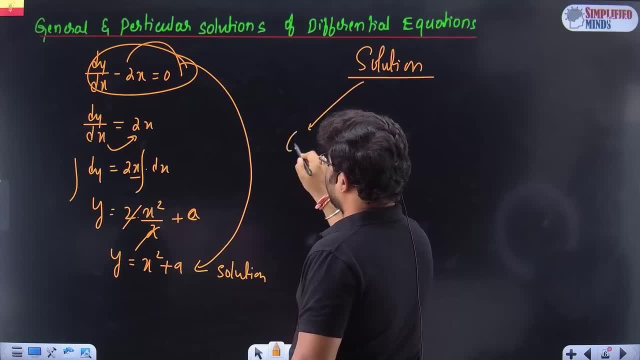 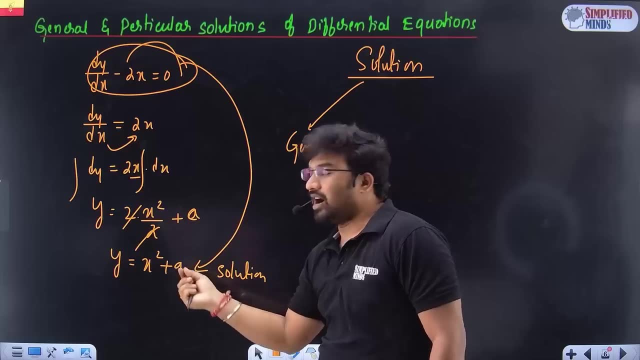 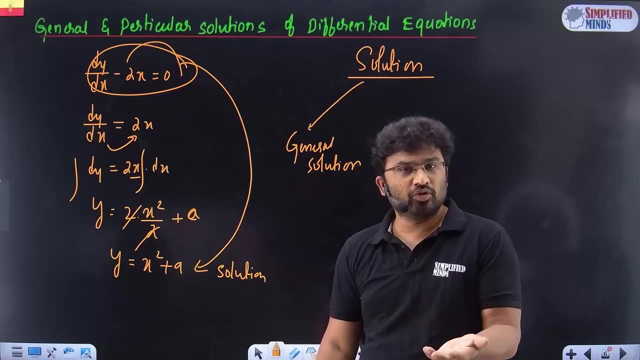 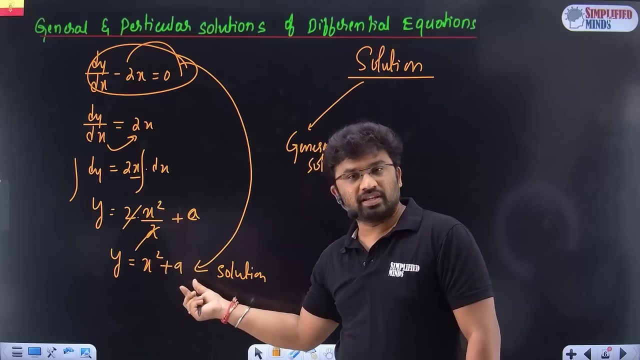 there is something called, as we have, general solution, general solution. general solution, the general solution, is a solution which is having some constants, like arbitrary constants, a, and with the arbitrary constant and then another can have anything you want here. y is equal to x squared plus two x squared plus three x squared. 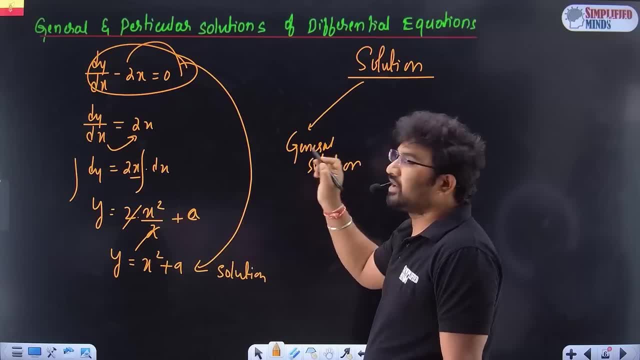 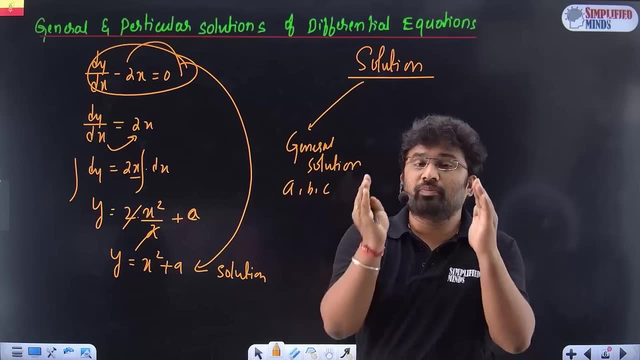 plus four. both. so general solutions are one which is having some arbitrary constants like a, b, c, d, another. actually a is equal to a sine x plus b cos x. now it's not a particular solution. you know, y is equal to x squared plus two, and that particular particular solution. 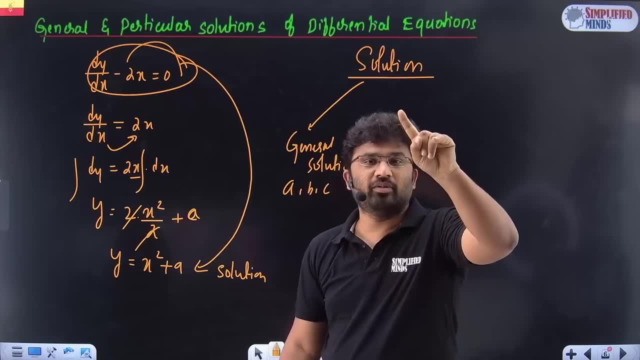 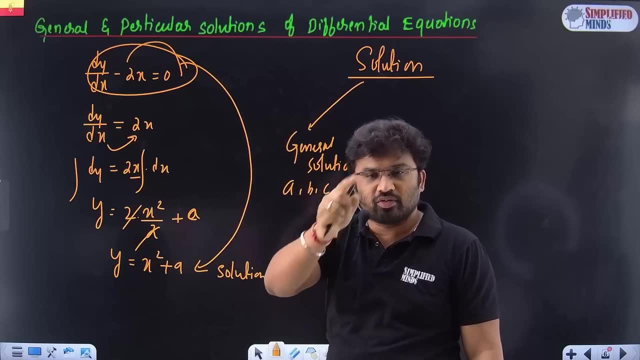 i would say that's the particular, that's the single parabola, x square plus a and a. i can keep changing. a is equal to a is equal to three. i'll get different family of parabolas. passing to the origin, you'll get like this: 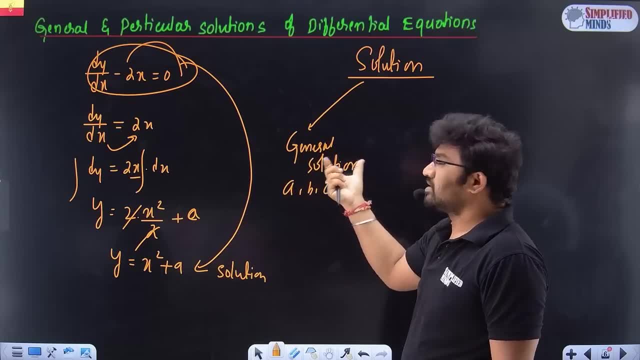 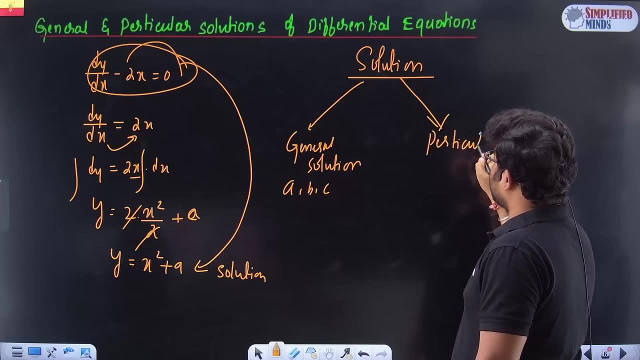 i'll tell you what i'm going to say. so general solution is an arbitrary constant a, b, c. here now, what is that? i mean? a particular solution, particular solution, particular solution. if you say a particular solution, so in that, in that there is no arbitrary constant zero. 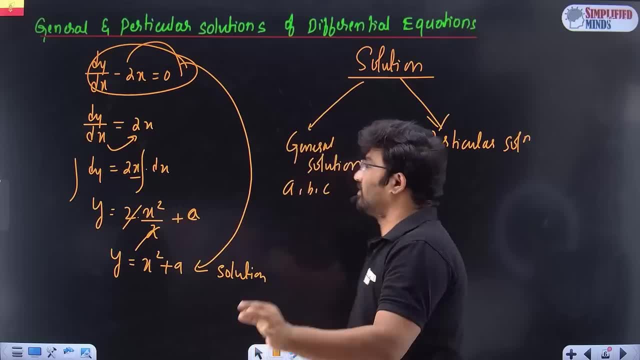 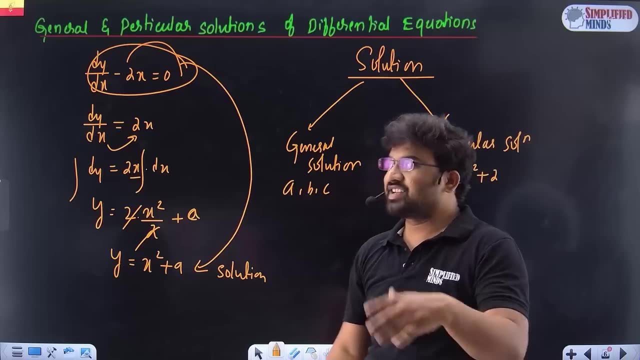 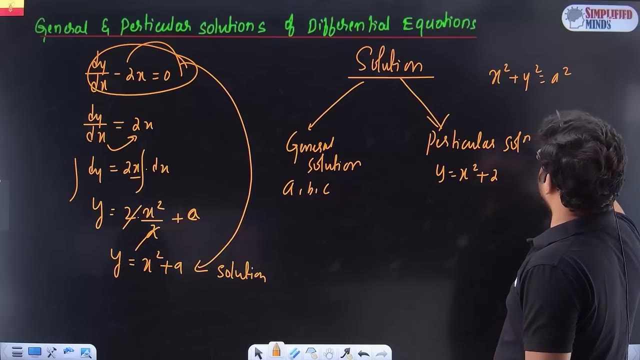 well, a is not there. a is not there. you particularly get the answer. for example, y is equal to x squared plus two. you get one particular solution in a general circle. let's see: x square plus y square is equal to, example, a square circle. what is this circle? a circle having center 0, 0, radius a, and what i'm changing is i'm going to be a 4. 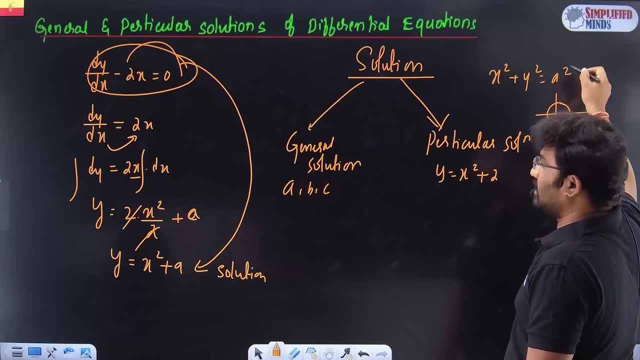 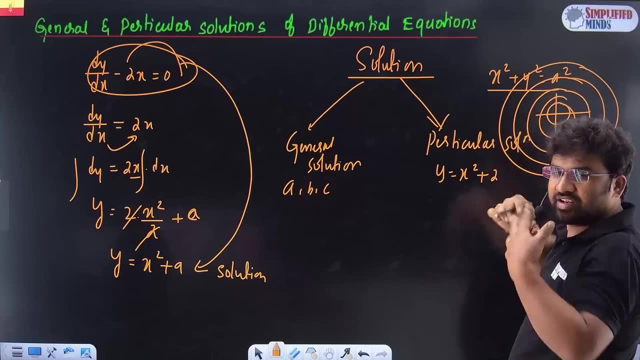 6, 8 or 3, nothing. i'll pay as 2, 3, 4, 5, 6, then you'll get family of circles, family of circles under the equation. it's a general equation. if i put, a is equal to, particularly in an, a and one. 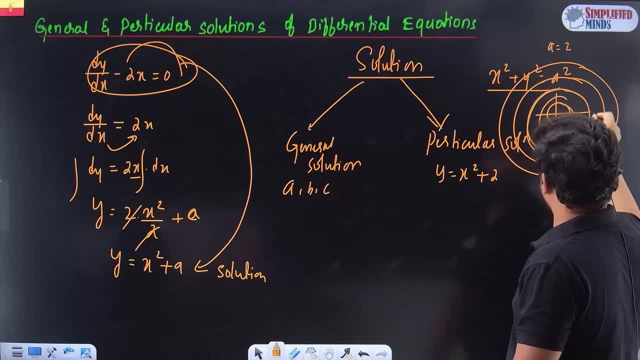 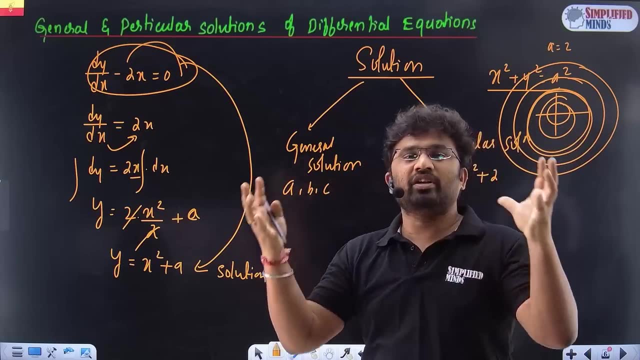 well, and two on top of that and part, i'll get a particular circle having radius only two, having send, having the origin zero comma zero. so when i say, when arbitrary constant is there, it'll give a family of curves, it'll give a family of curves if you want to find a particular. 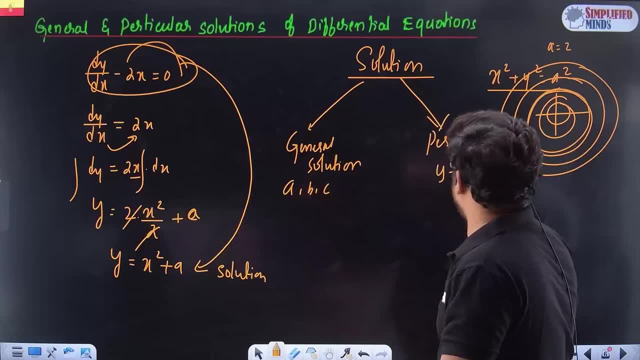 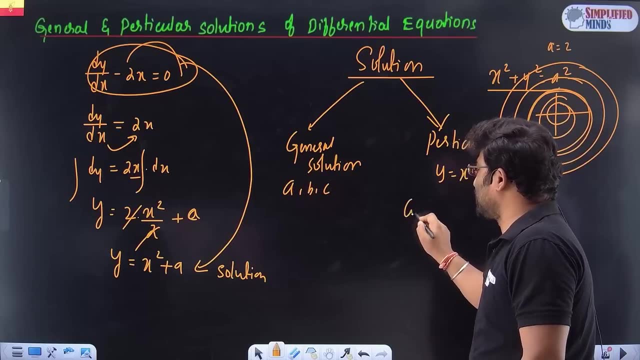 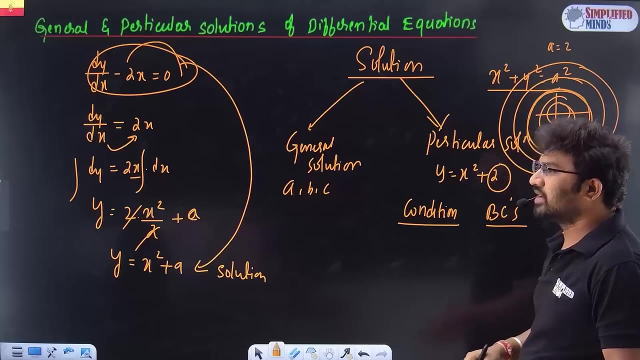 solution for that a particular bacon trailer. you have to find that arbitrary constant of fine model there then. hey, arbitrary constant of fine model, though they will give conditions, our conditions, or boundary, we call boundary conditions bc's and the healthy boundary conditions in there they'll give some conditions. what's the condition at? x is equal to y. much for. 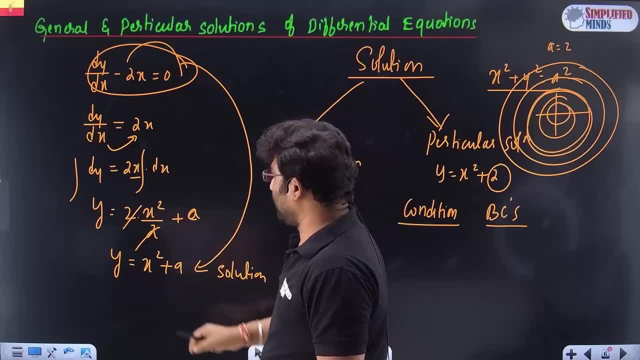 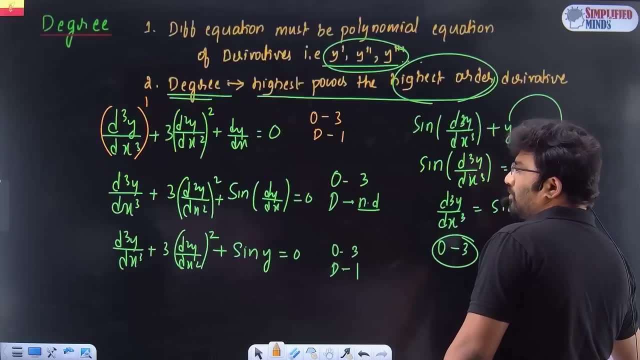 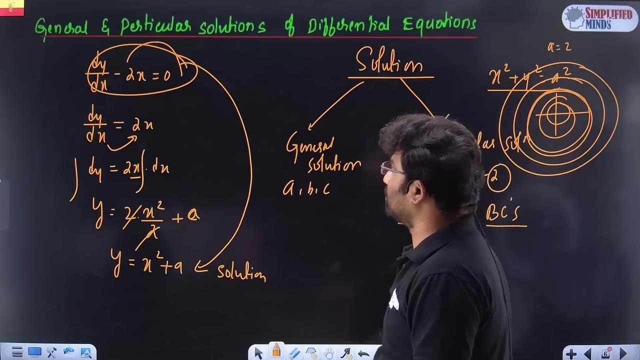 example, the question. again, i want to actually find what the question actually was. uh, the question was actually plus two alva, so i don't know whether it's a plus two. now the question: i'll give conditions nine, but i'll give conditions and actually question one, though y is equal to x. 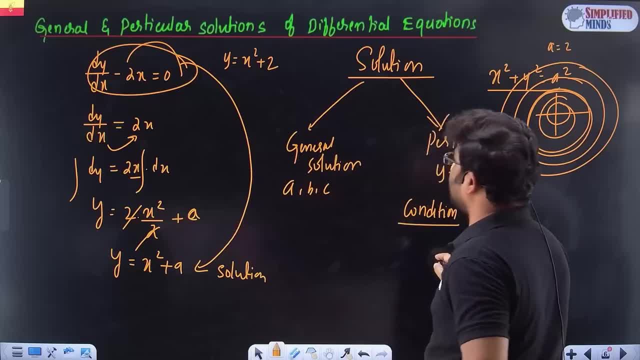 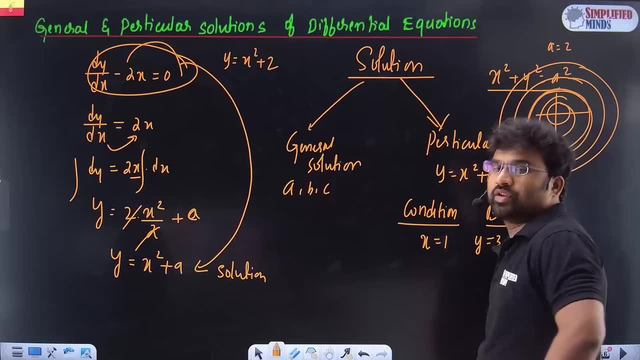 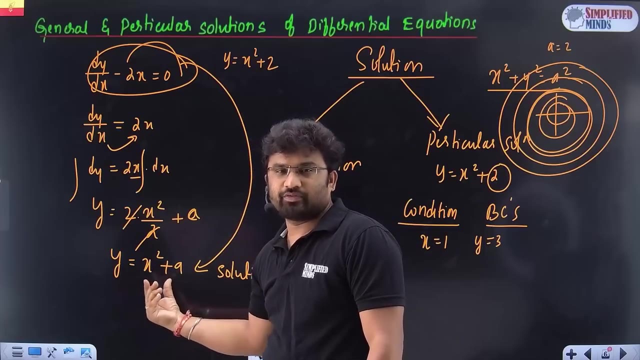 square plus two alva. so condition, condition when x is equal to one, i mean x is equal to one, y is three and the condition. so now, when marbeco, now differential equation, is solved- i'm going to, you'll get a solution- y is f of x. 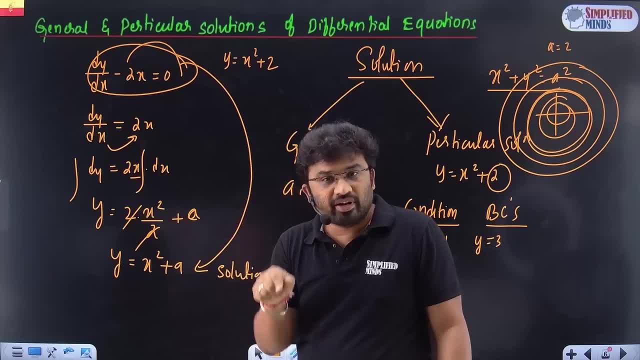 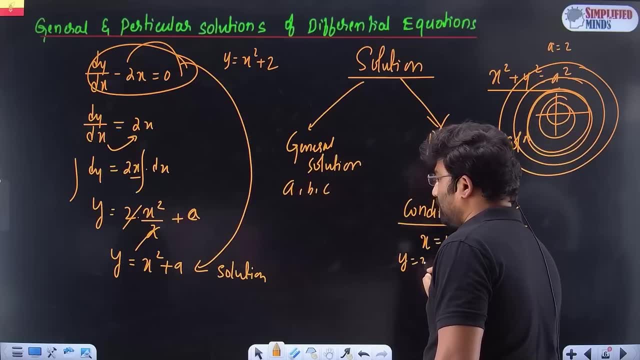 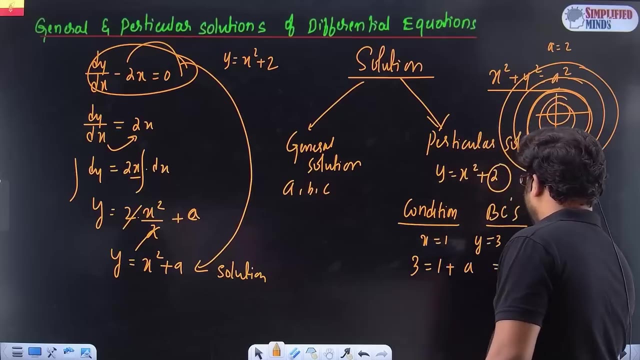 so i f of x. yeah, a value, delva i a value in fine model condition code written in condition: when x is equal to one, y is equal to three, and substitute one another: y is equal to three and x is equal to one and three is equal to one plus a bar, then you get a as two, so your your particular solutions becomes. 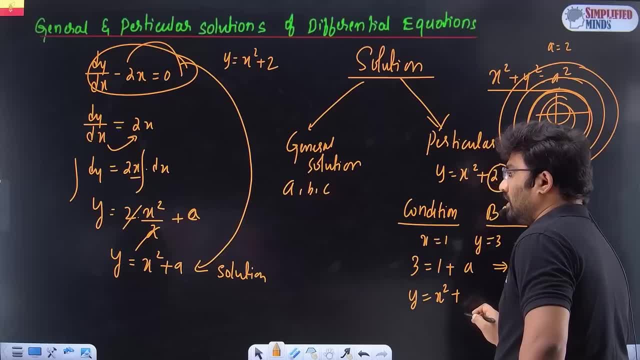 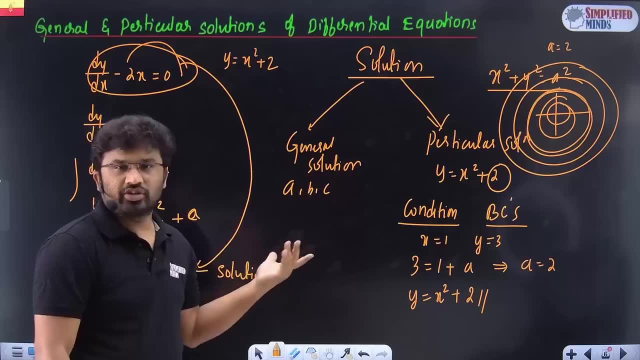 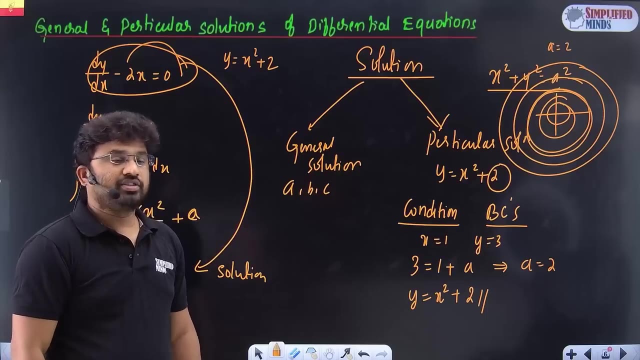 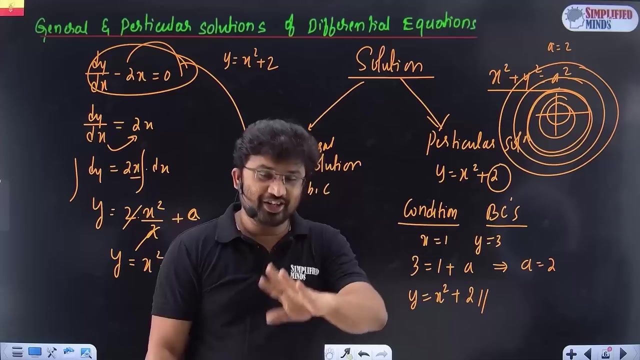 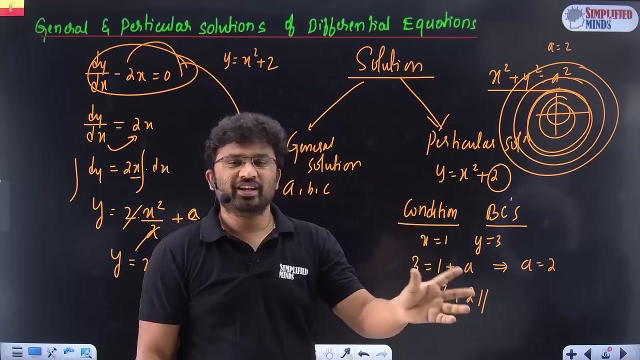 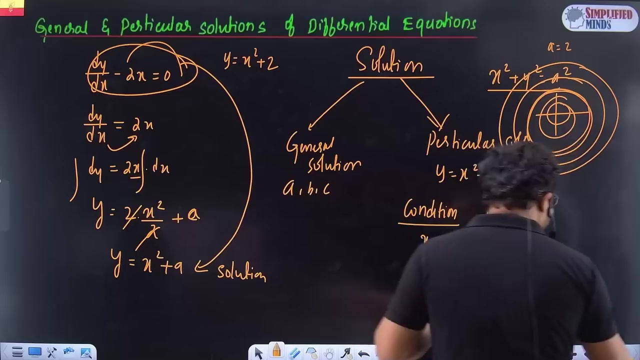 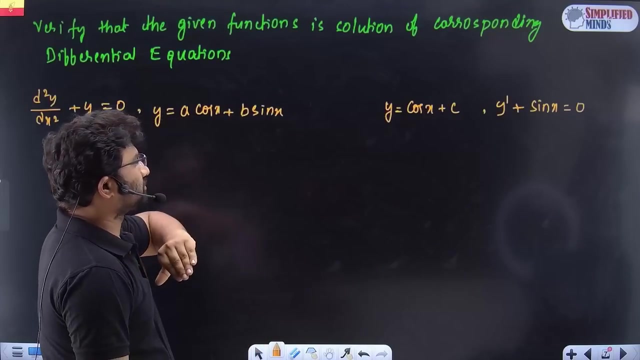 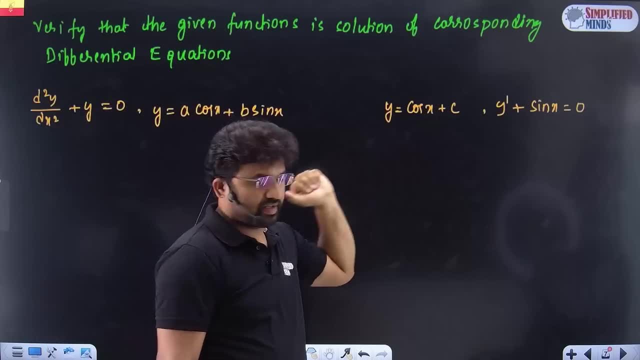 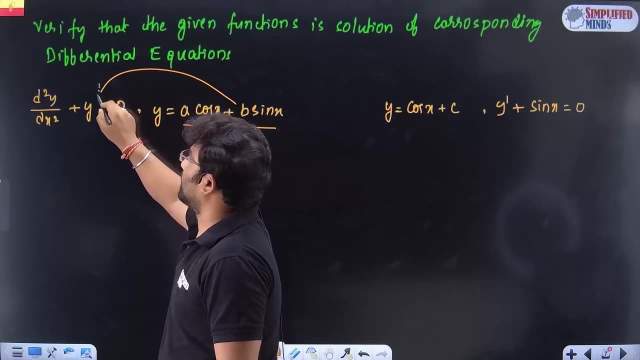 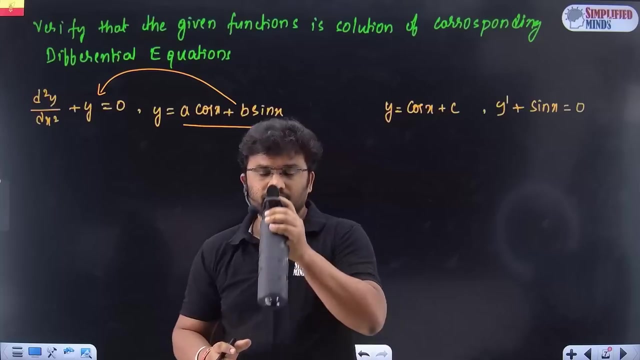 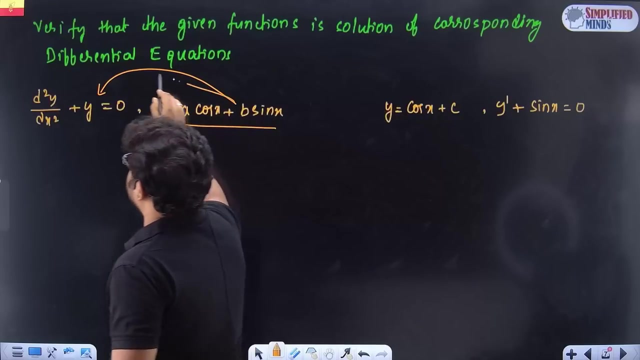 of corresponding or not. After that, forming differential equation is given. So it is simple. So you have to take this value and substitute it here and check whether it is a solution or not. Do it by yourself, You do it. So now you have to substitute here. 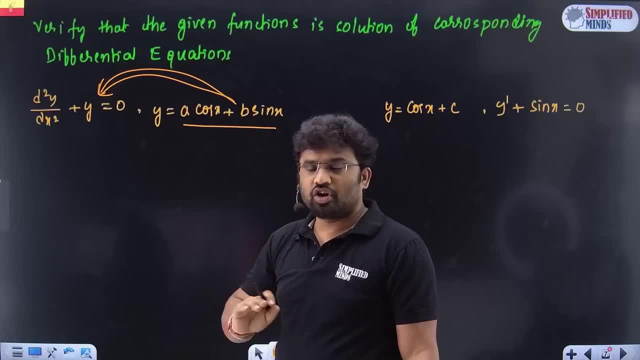 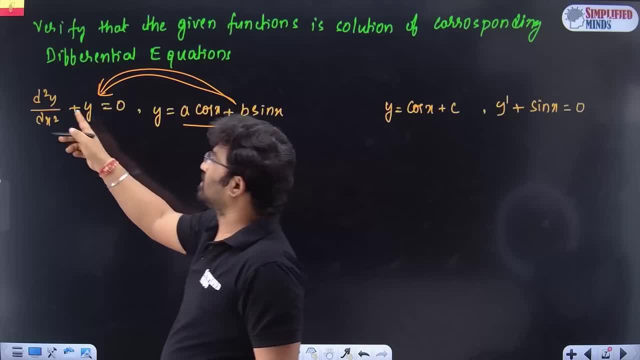 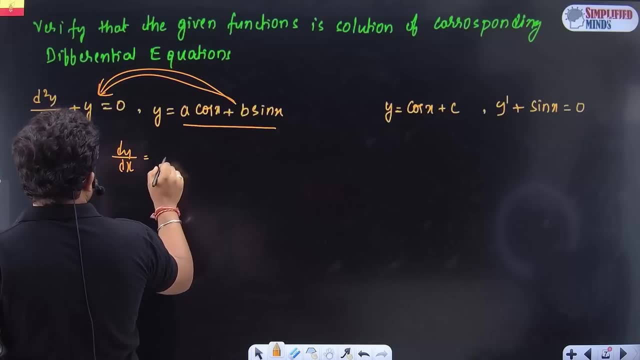 Because there are arbitrary constants, are there. If you do not substitute this, you will not be able to differentiate. Obviously the answer is not there. So dy by dx. The differentiation of a is cos minus a, cos x plus b, into sorry sin x Cos differentiation. 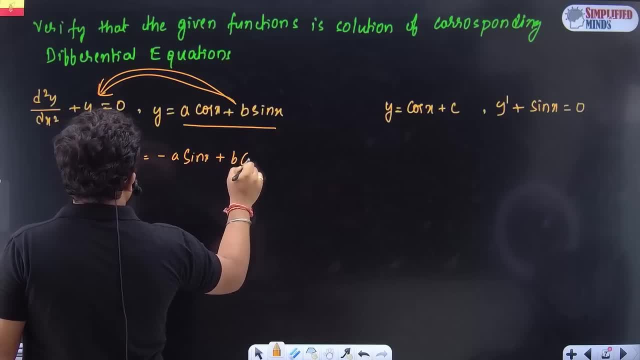 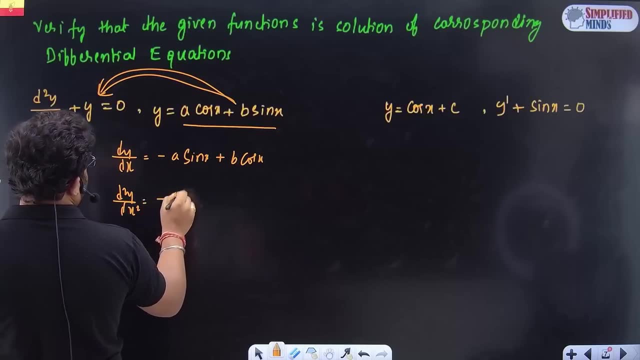 minus sin x plus b into sin x. differentiation cos x. Is it clear? Again, I am differentiating d square by dx square. When minus a is like this: sin x. differentiation cos x is like this: b cos x, cos x. differentiation minus sin x. So minus b sin x. So obviously. 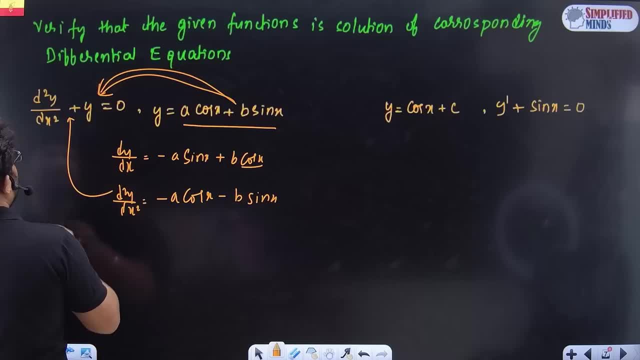 if you substitute it here, the answer will be 0.. Because d square by dx is this much, We will get negative. But y is positive, It will be 0.. If you substitute there, we will get minus a, cos, cos x plus b, sin x plus y Plus y is just an example. It is simple. 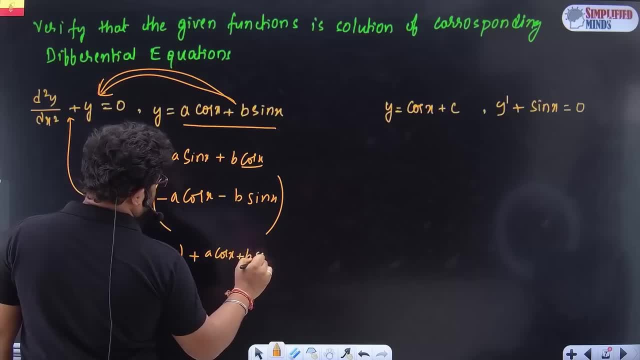 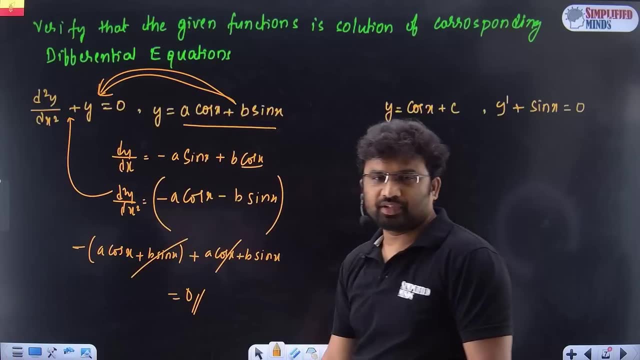 It is nothing to do too much. a cos x plus b sin x is 0. So obviously all these two are cancelled and your answer is 0. Therefore it is satisfied. It is a simple question. Understand Then again. y is equal to cos x plus c y. double dash, again same Differentiate. 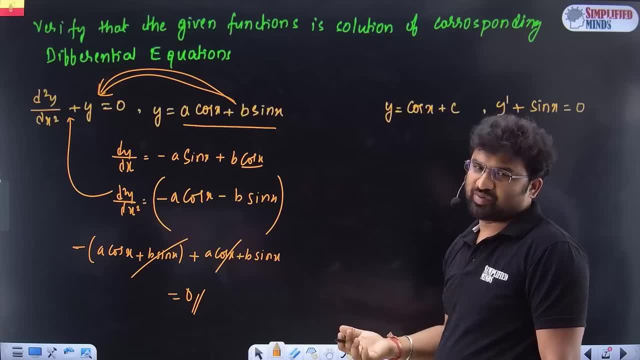 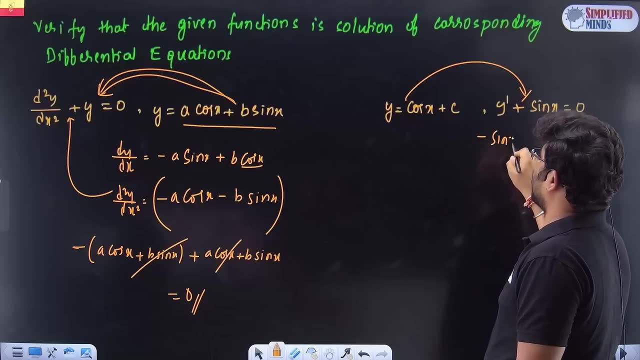 it Simply. I am beginning the differential equation. Substitute it, check it and the answer is same. Because y cos x, y dash differentiation is minus sin x. C differentiation, constant differentiation, is 0.. Minus sin x, plus sin x. Therefore, it will become basically 0. 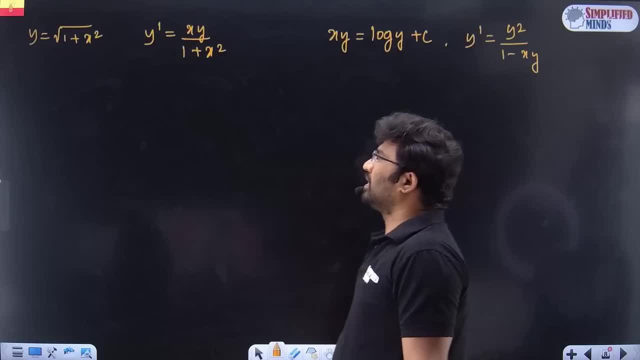 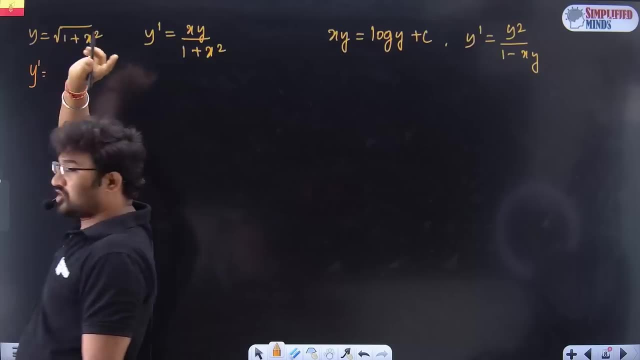 Understand. So let us go for next questions. This is simple: y is equal to root of 1 plus x square y, double dash. Find it Now. find it: Y dash differentiation. So in the first lecture I told you something: chain rule. Do you remember What is root something 1. 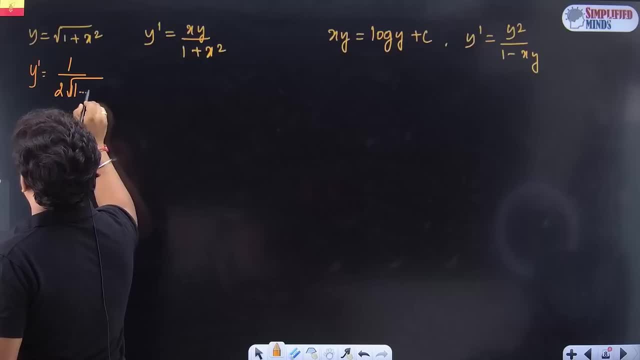 by 2 root something. Do not forget What to do next. Again: differentiate the inside function. Then you have to keep 2x there, 2 to get cancelled. Then you are going to get x divided by root of 1 plus x square. This. 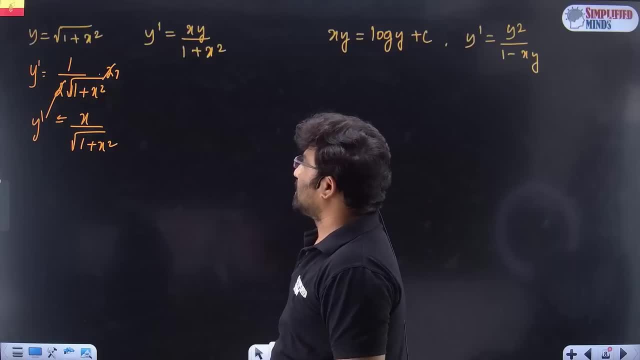 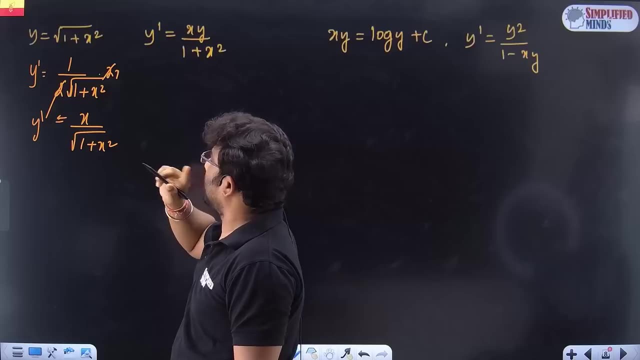 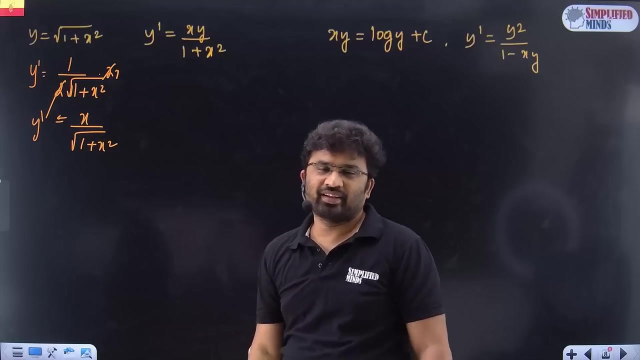 is y dash. So, Kelvin Sethi, now you can continue this In y dash substitute. simplify again your substitute here you will get both cancelled. But now I can get from here. only we can get this also. We have come to y dash. x divided by root of 1 plus x square. What is the question? 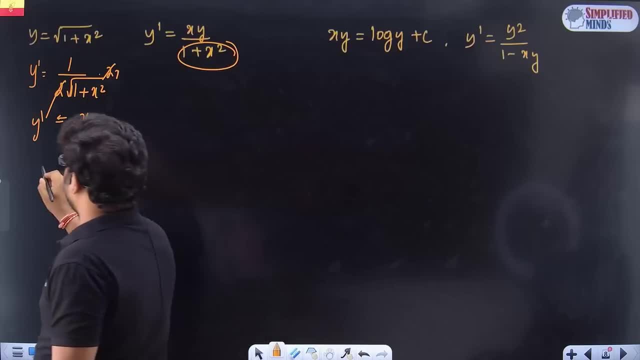 there Is there a big 1 plus x square. What to do next? There is y dash right. What will I get excited about that? Divide by root of 1 plus x square. no, there is sin of 6. There. 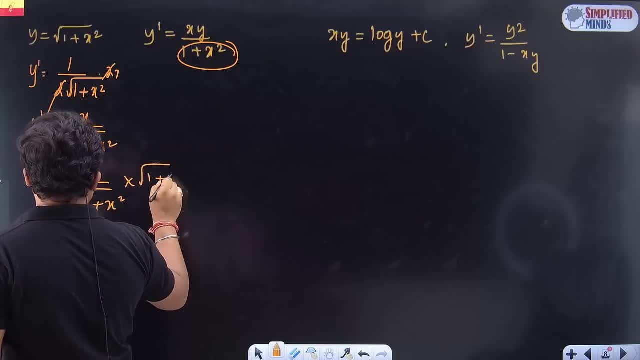 will be Well Gingerider. and then there is y dash, twice step, and both For the sake of complexity. look for solutions. So get rid of the Aryan, the OU word I made earlier. For the sake of complexity. look for the мощeter formula, if there now. 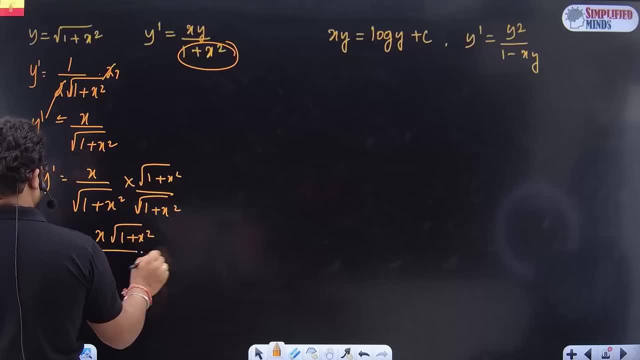 there is none except for the day but one. But if you look at trick here, so x divided by root of 1 plus++ by root of 1 plus x square is 1 plus x square divided by root of x squared. x squared divided by root of x, I think x is square. So that is this will be x into. 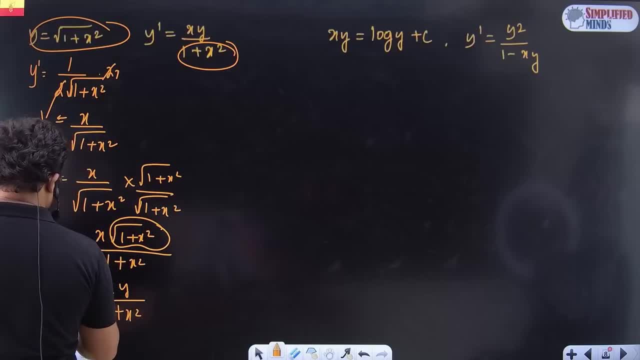 root of 1 plus x square, divided by root of x square. So this is y dash. So what is my root of 1 plus x square? There is nothing but y, So answer is basically xy divided by it. from here we started from this and we got this answer, so therefore it is satisfied. it is. 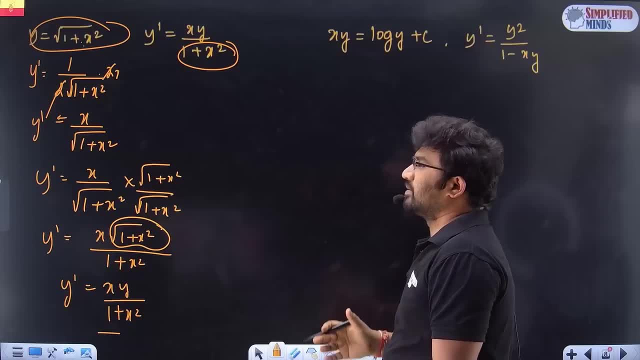 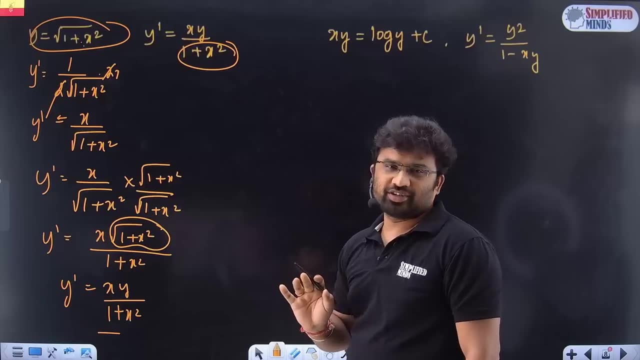 a simple level as these are the questions are not in new simple questions. let me exercise 9.2, only 9.1. all the order and degree: 9.2. check my name in ncr: exercise. all these questions are very simple. you don't care about board exam. only next: x, y is equal log y is equal to c lva. 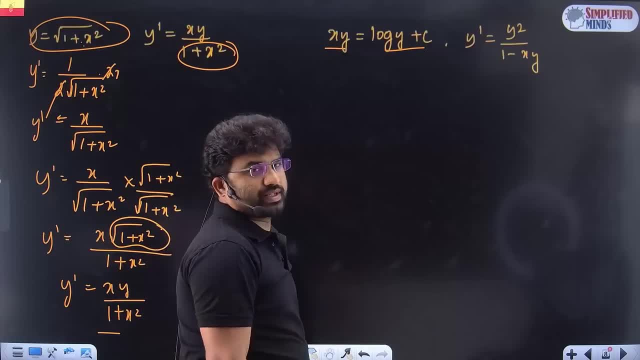 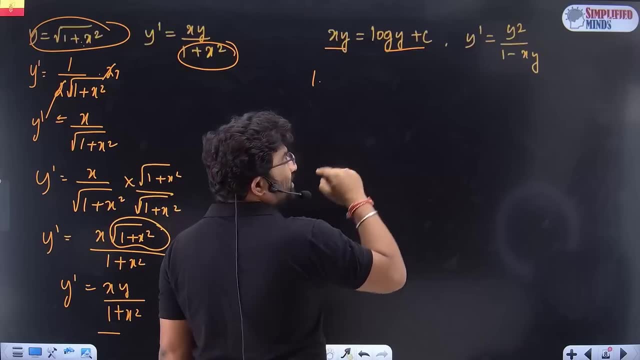 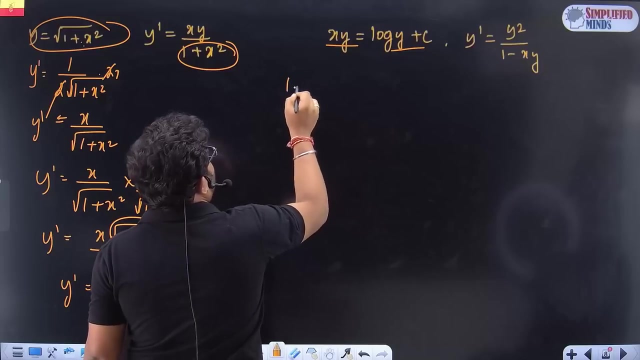 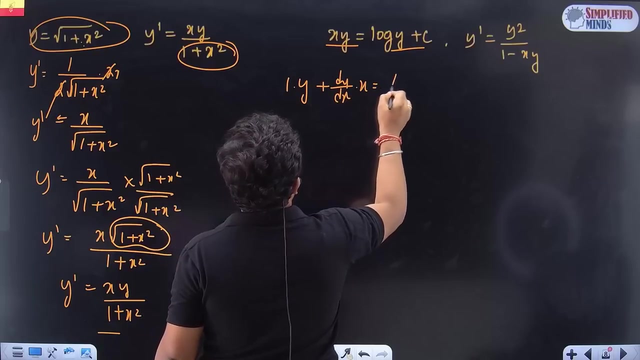 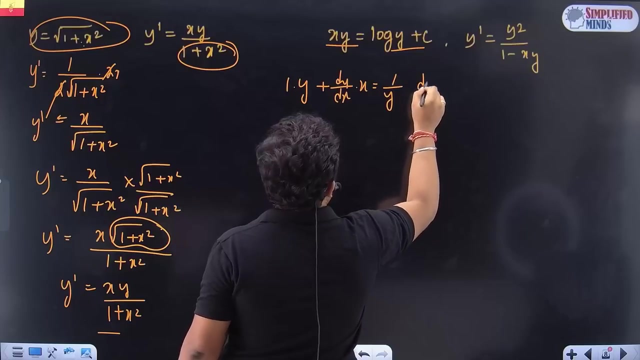 you should do by yourself. x differentiation of the one, why not? uh, you remember this. this is called as implicit function differentiation and first lecture i helped you didn't again. y differentiation, d y by dx, log y differentiation, you know, one by y into dy by dx. in first two, differentiationally d y by dx, constant differentiation, zero, that well you. 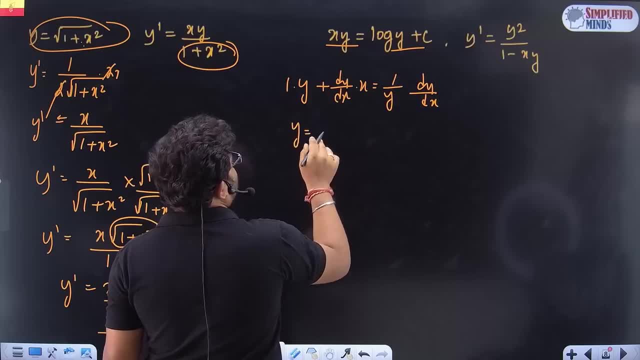 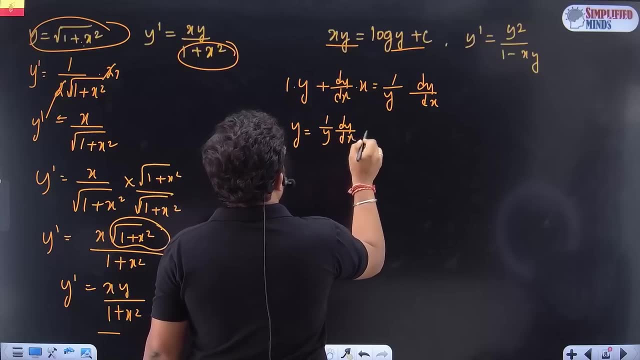 can shift it and get the answer. but i think you'll get the answer. so y is here, shift my d y body is outside, so you can shift my laga and then you get 1 by y into d y by dx minus d y by dx into 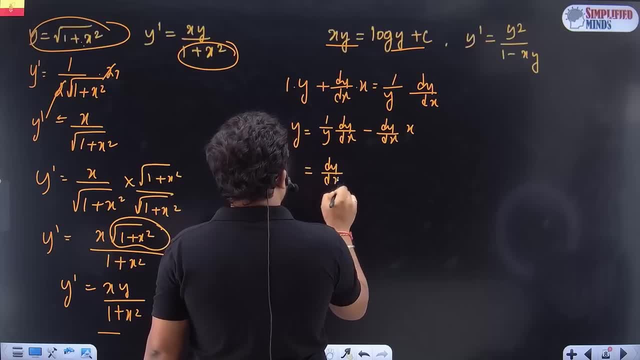 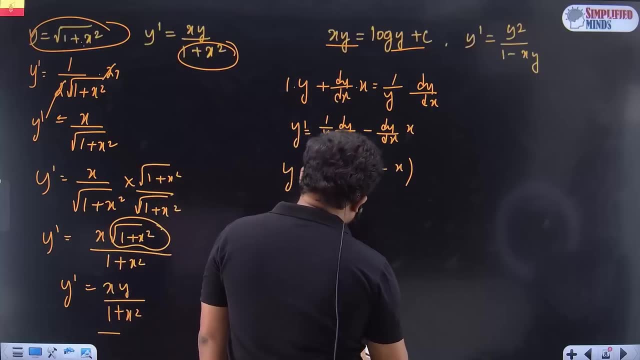 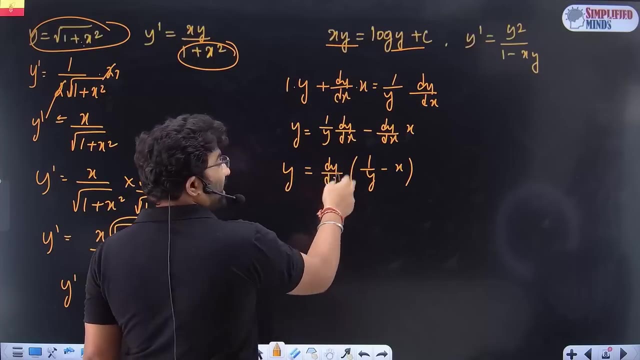 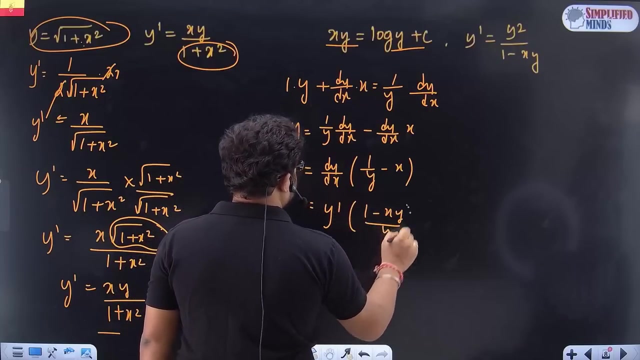 x bertha, non d y by dx i will get 1 y y minus x bertha, that's equal to y. so y dash lva. this way it is divided by y equal to y. if this y, this side, you will get y square equal to y. dash into 1 minus x y. 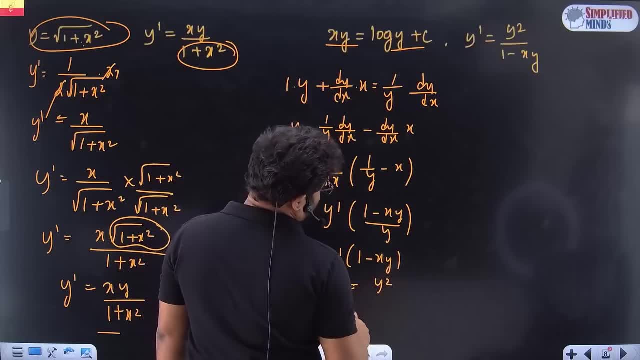 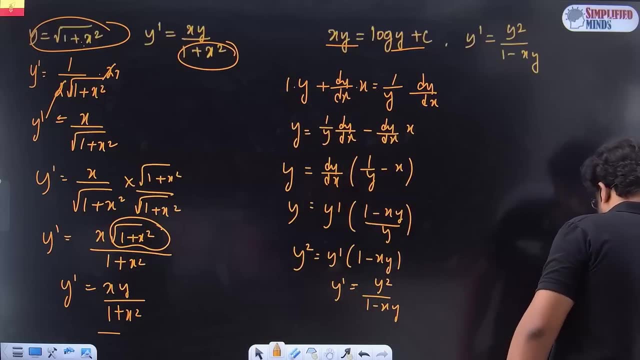 what is my y dash will becomes y square divided by 1 minus it. i don't know, it is easier. you can just directly prove it. it's very simple, okay. so you lecture early what i have done. so i have. that's all, yeah. so other thing, you mean ncr to? 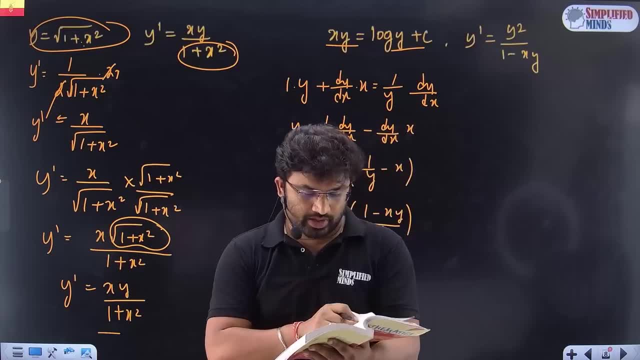 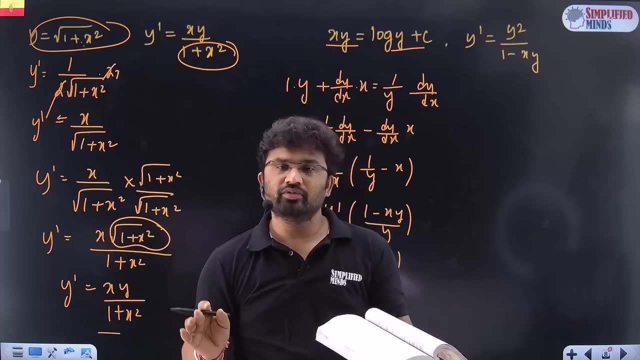 check my border, ncrt, ncrt early. so i've just given all the degree with the order: 9.1, 9.2, full. check my body in law. questions on you would solve my body. so you're ready. so you're ready so that my 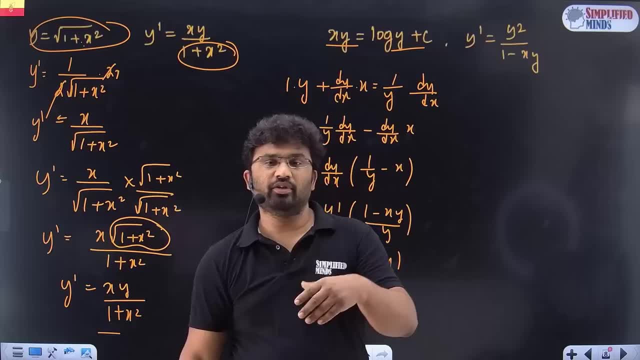 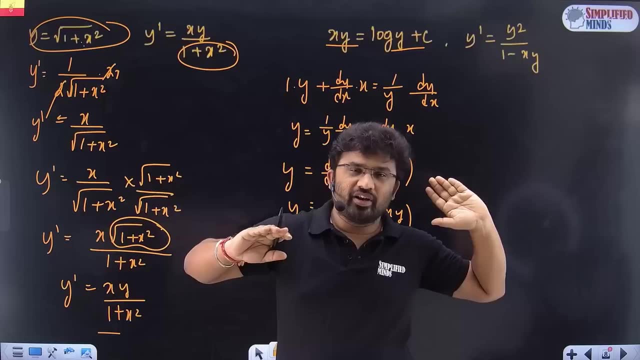 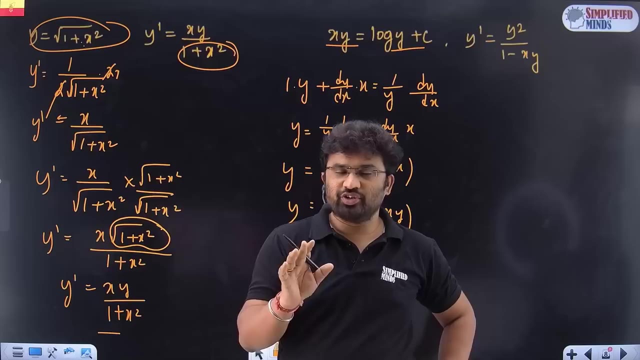 next will form: uh, for me differential equations or beta directly. we'll go for the solving differential equations, i'll leave them and i'll end up from my questions about the basics. so so, if you go one order, one order, you know. if you go in order, you order study mark. so that's it. i hope you understood. 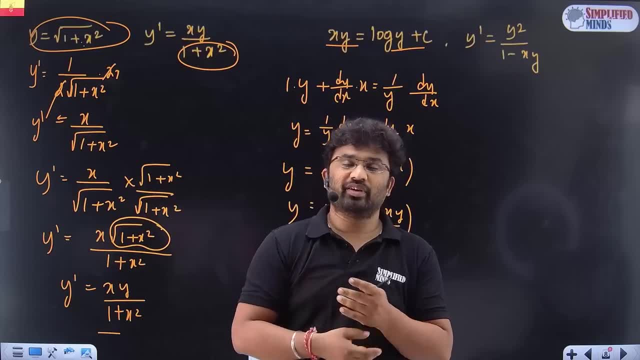 it's a very small lecture next on a differential equation solving. it'll be very nice and see you there and bye. bye, take care.